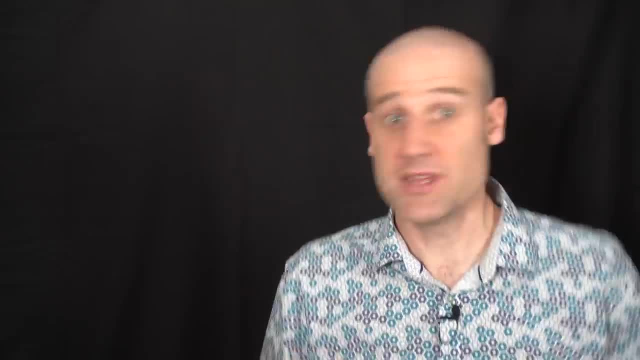 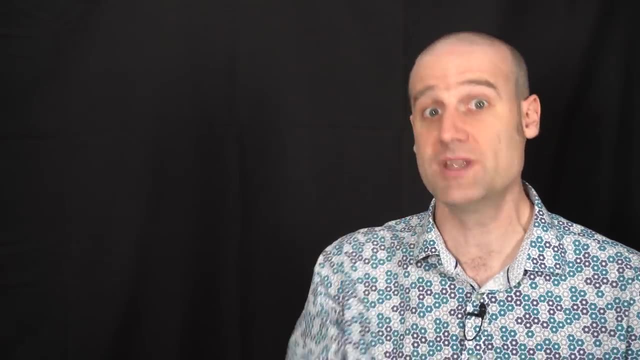 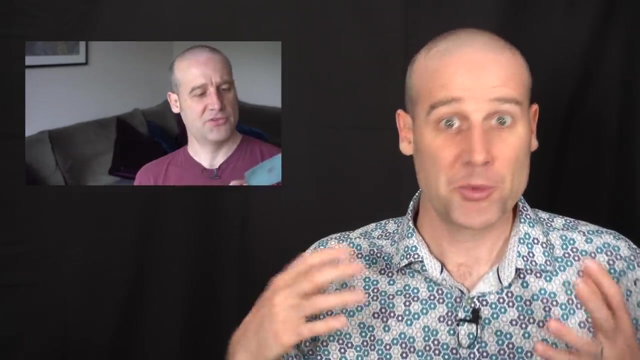 in both directions. most people just don't think about negative valued Fibonacci numbers. and as a bit of an experiment, because I was curious, I had a puzzle recently on my separate series of videos- Matt Parker's mass puzzles- where it was a Fibonacci style problem. people had to submit two starting 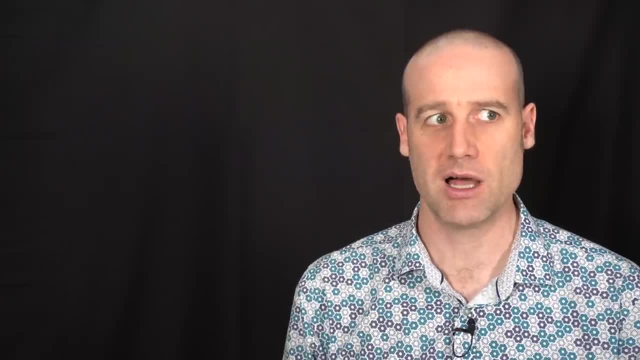 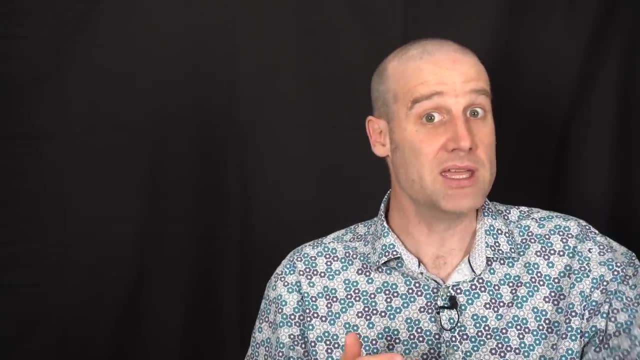 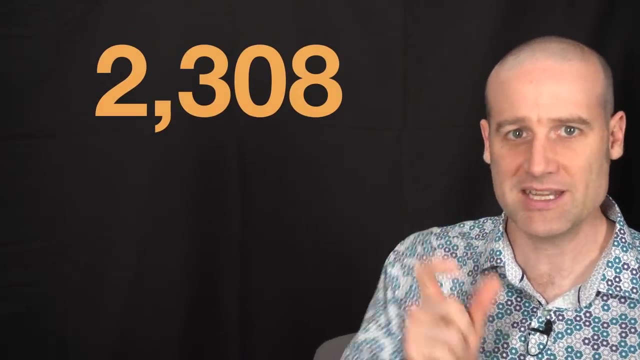 values of that kind of sequence- and while I didn't heavily imply you could use negative numbers, I did hint they were possible and arguably they were the better solutions to the puzzle- and of the over 2000 valid starting numbers for a sequence that different people sent. 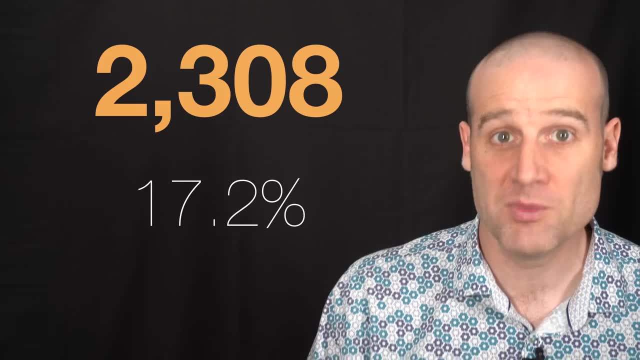 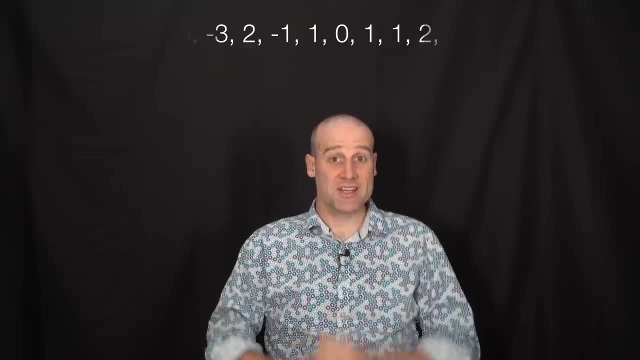 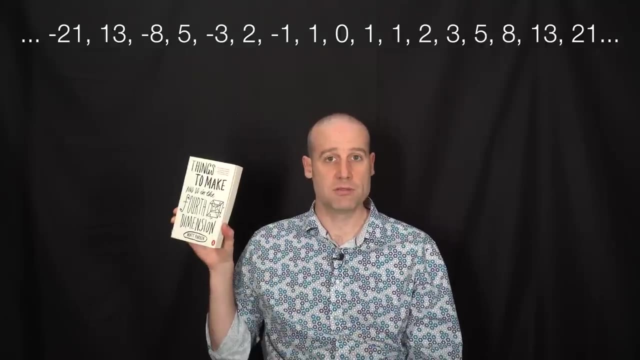 in. only 17.2 percent of them used any negative numbers, so most people just didn't cross their minds. so there you are: you can extend the Fibonacci sequence in the negative direction. I actually wrote about this several years ago in my book things to make and do in the fourth dimension, and 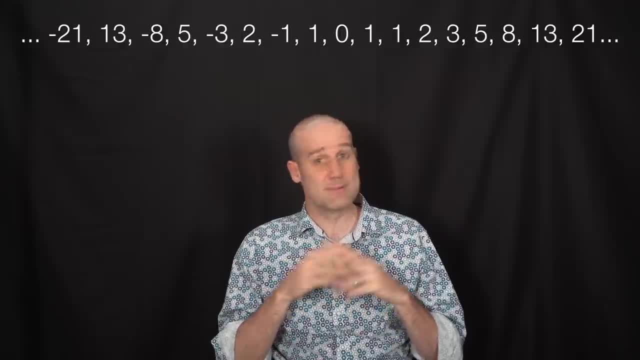 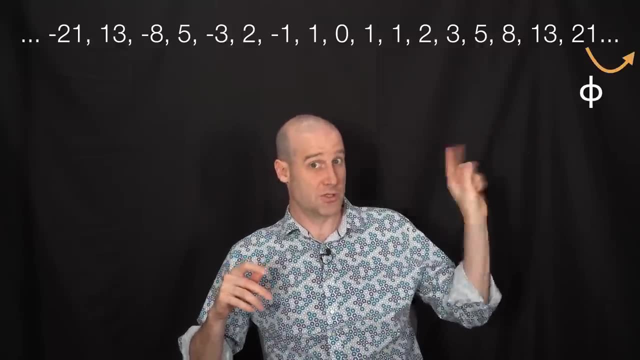 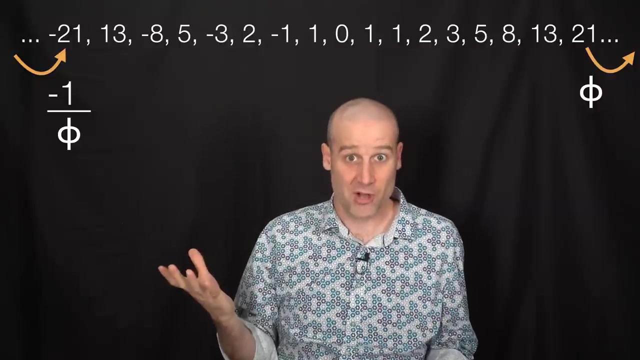 there's a few interesting things about it. so some people may know if you look at the ratio between two terms in sequence, going in the positive direction, that approaches the golden ratio. if you go in the negative direction, it approaches the negative of the inverse of the golden ratio, which is kind of fun, and the numbers 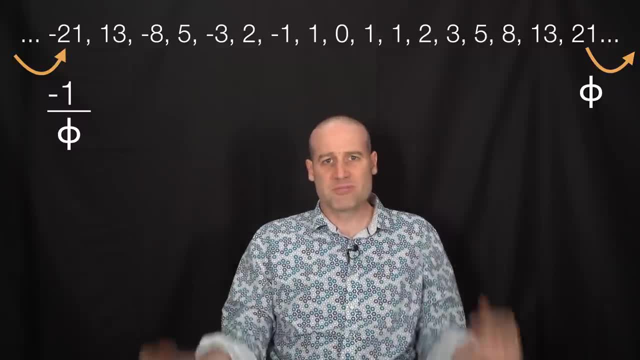 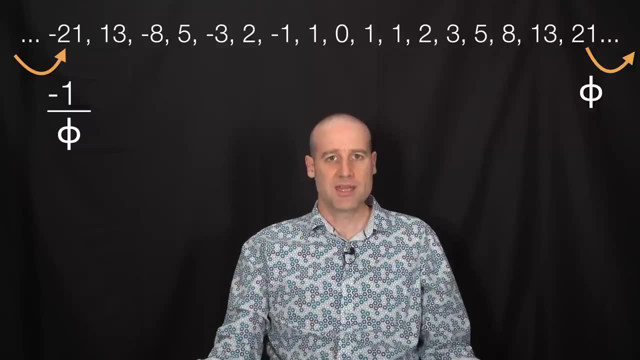 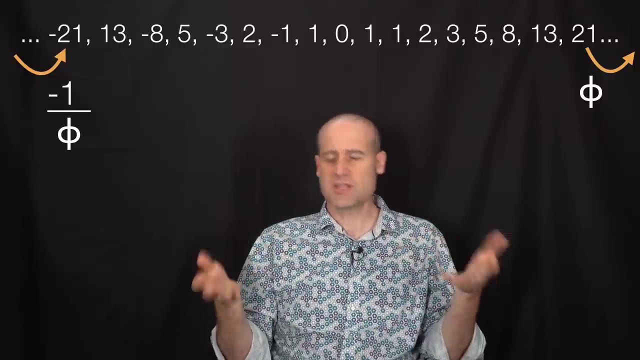 are the same, but they alternate positive and negative. and you know what? I wrote a little bit about some of that stuff and then I kind of, you know, filed it away. mildly interesting, but not astounding. however, I was thinking about this puzzle and I suddenly thought: hang on, are there any other interesting? 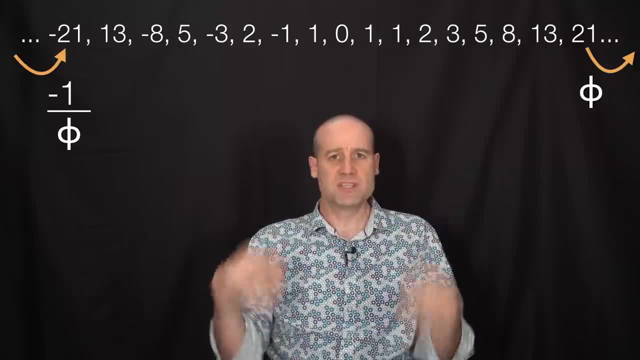 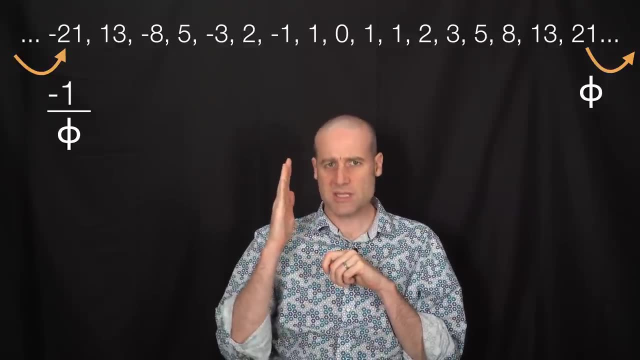 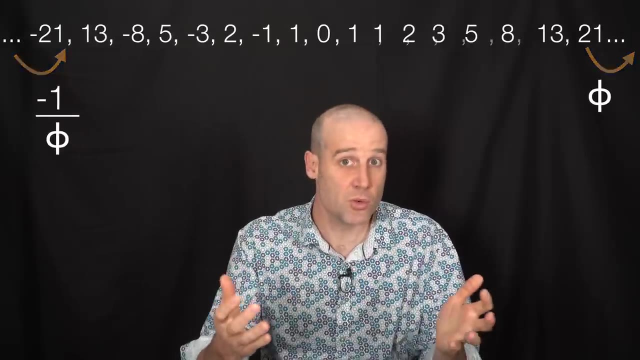 things about how we can extend the Fibonacci numbers. I went through the stuff I'd done before and I went hang on a second. I've only ever looked at extending it in terms of discrete whole numbers going in both directions. is there a way to fill the gaps? and there is a. 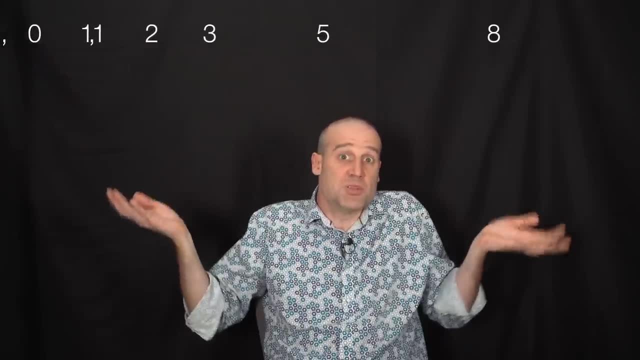 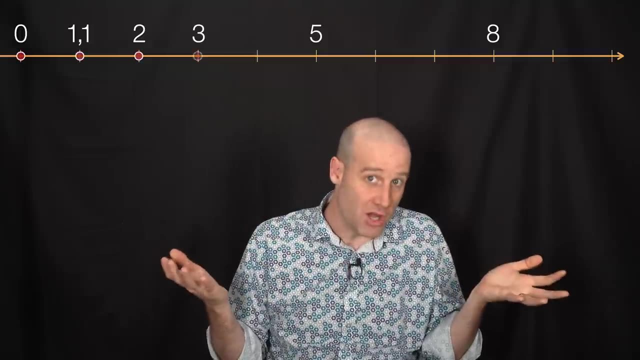 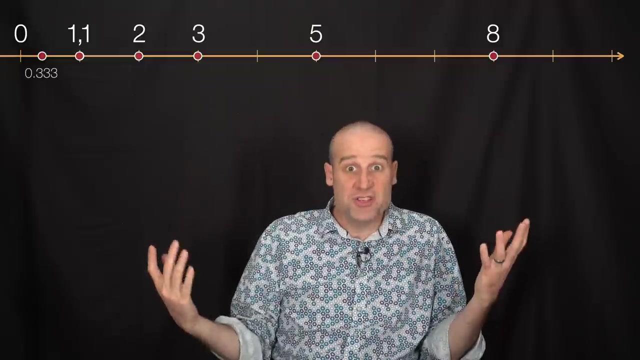 trivial way to do it: you can just take points that are in between. so if, instead of adding whole numbers, if you imagine them on, let's say, a number line, you can go part way along. so if you go part way between zero and one, let's say a third, but it could be, you know, three, sevenths a pi. 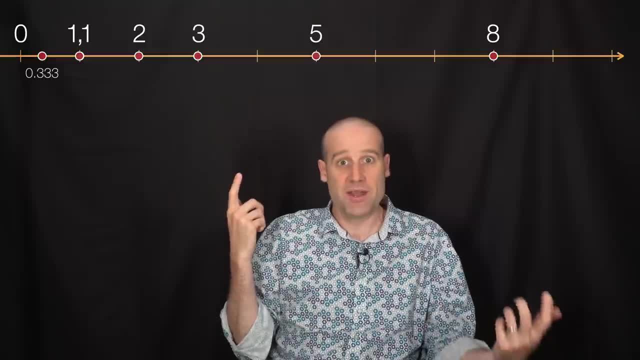 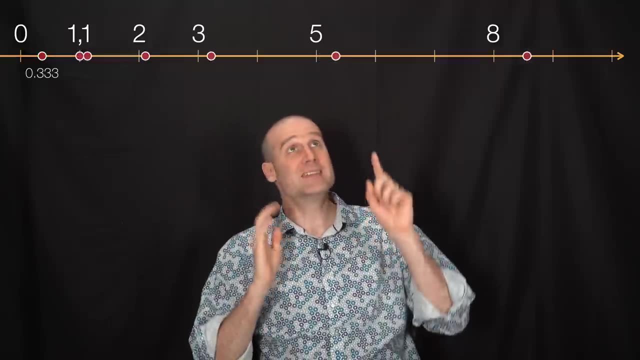 whatever you fancy you then. well, the next one, because you've got those two ones together, there's no points between them. you always have one for the next term, and then you'll actually hit the same ratio all the way along. and because that works for any real number in the first range, 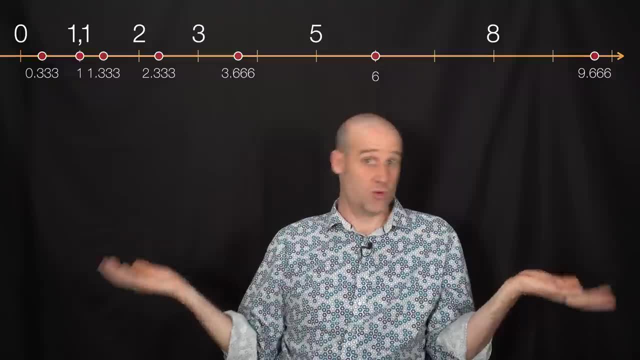 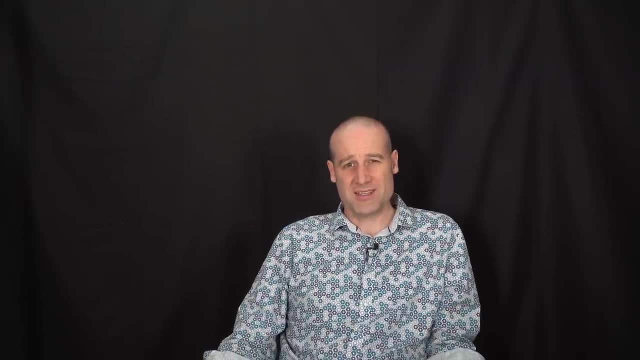 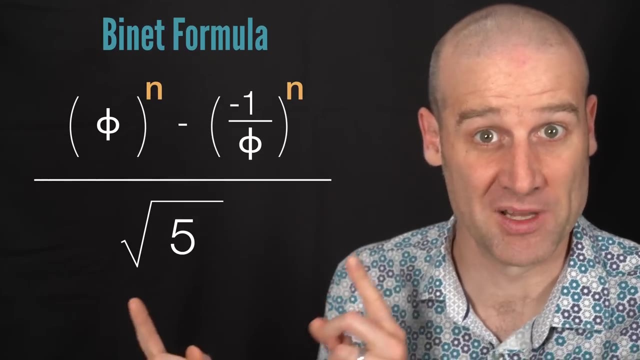 you can include any arbitrary point on the real number line in a Fibonacci style sequence, but it's not particularly interesting or exciting. but then I remembered something else. I had remembered this: the Binet formula. now, I've talked a lot in other videos about how you can generate things. 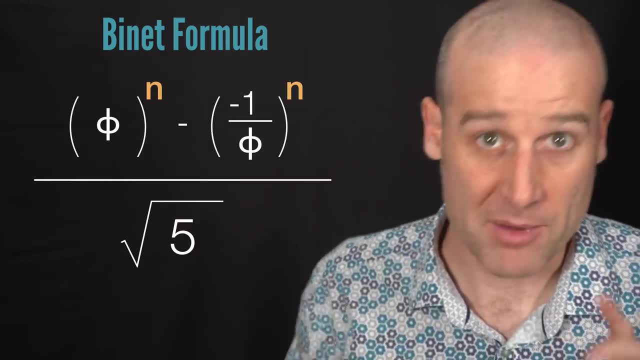 like the Fibonacci and Lucas sequences. I'll link to them all below. but I have not mentioned the Binet formula and it does look a little bit like the Fibonacci formula. but it does look a little bit like the Fibonacci formula. but it does look a little bit like the Fibonacci formula, but it does look. 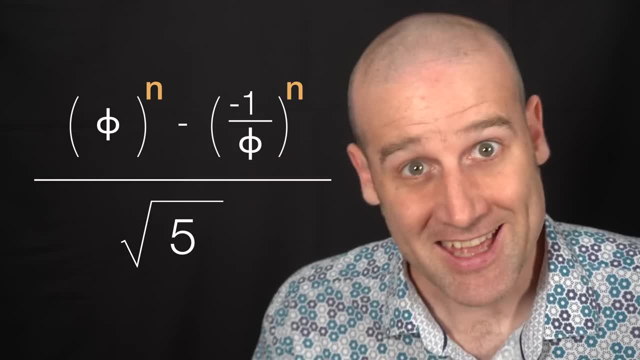 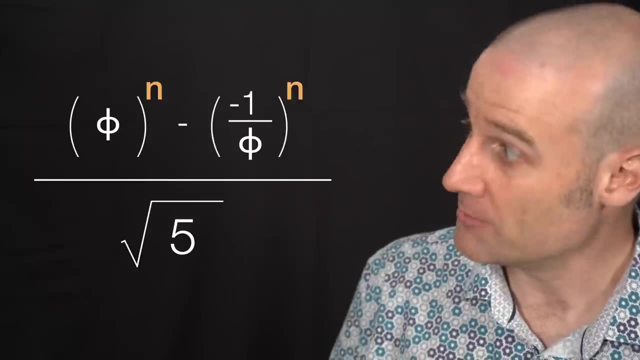 like the Fibonacci formula, but it does look a little bit like the Fibonacci formula but it does look very, very Fibonacci e. it's got the golden ratio to the power of n, it's got the negative inverse of the golden ratio, also the power of n, and of course you're dividing it by the square root of 5. 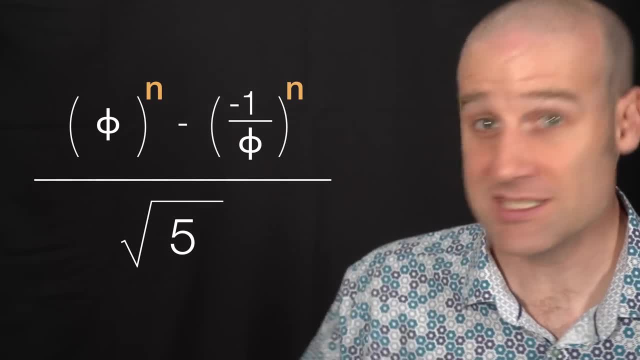 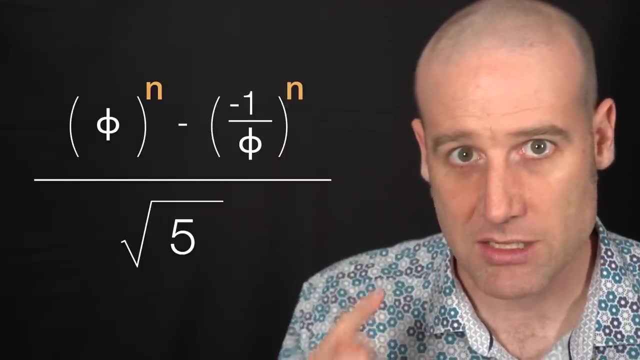 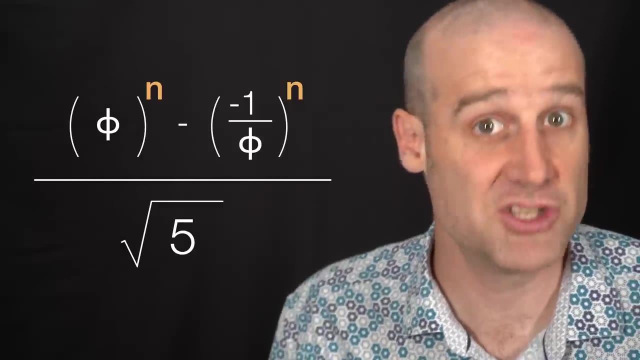 big fan. links to other videos below now. this formula is amazing because if you put in any value of n, it will give you the nth Fibonacci number. it doesn't just work going forwards. if you put in n equals zero, you get the zeroth Fibonacci number. if you put in n equals zero, you get the zeroth Fibonacci number. 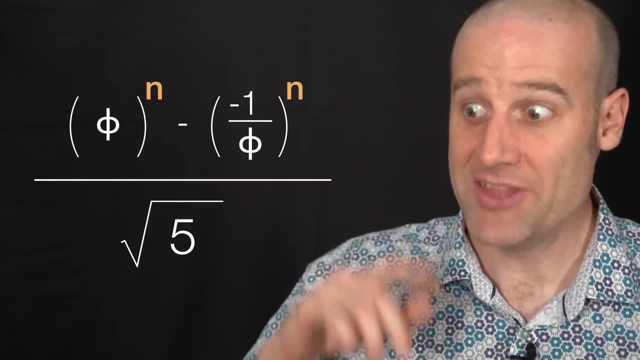 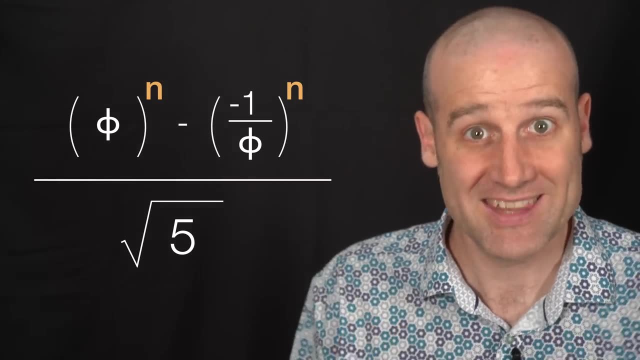 zero. if you put in negative values of n, you get the negative Fibonacci numbers. it works perfectly forwards and backwards and I thought you know what. I can use this to try and fill in the gaps. what happens if we don't put in a whole value of n? what if we put in 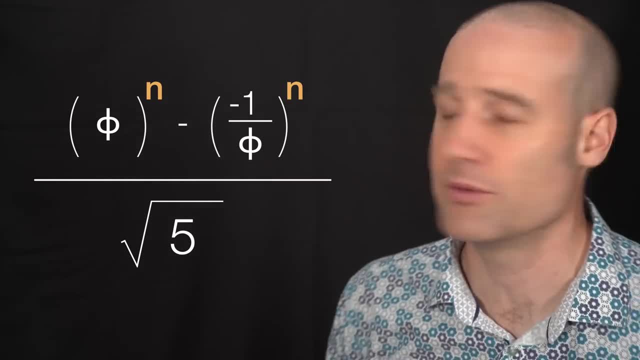 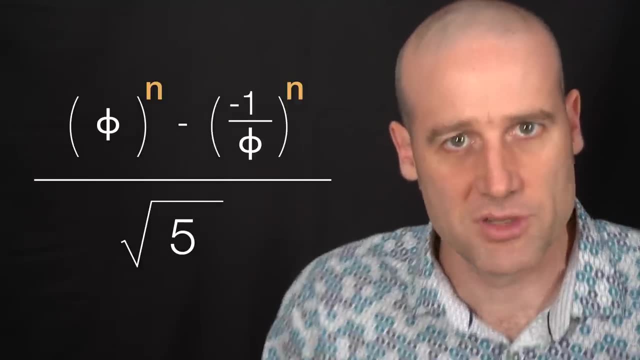 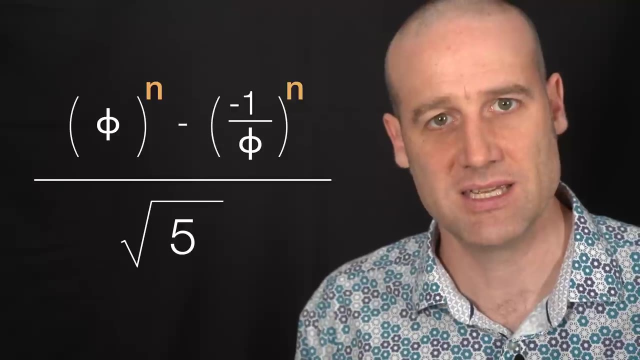 a fractional value of l how the way that's not gonna work because you can see there's a negative number there, negative of the inverse, the golden ratio, that's a negative value. and if you raise something to a fractional value, that's effectively taking a root. and, of course, 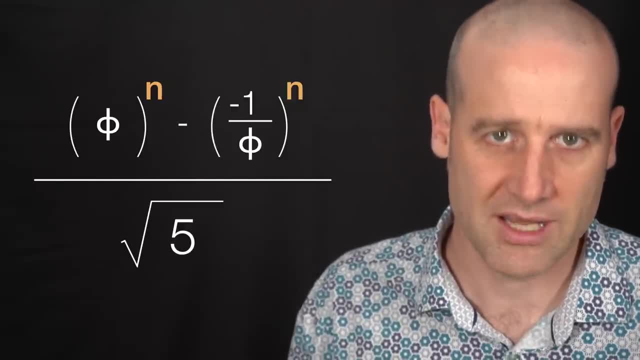 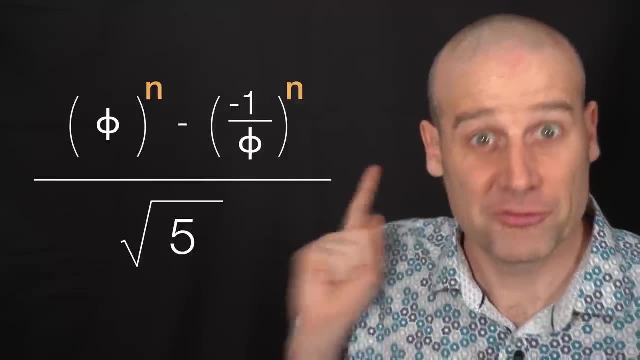 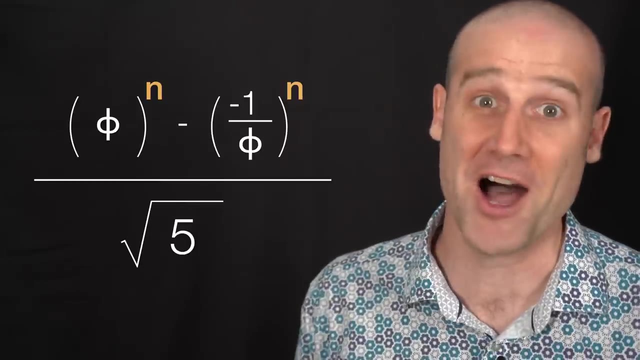 you can't have the root of a negative number unless you allow complex results. if we put in the fractional values of n to get the in-between values in the Fibonacci sequence, we're going to get complex results. I was so excited when I realized this and I did it initially just for. 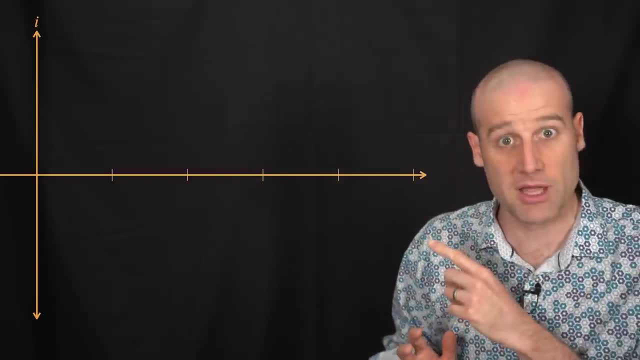 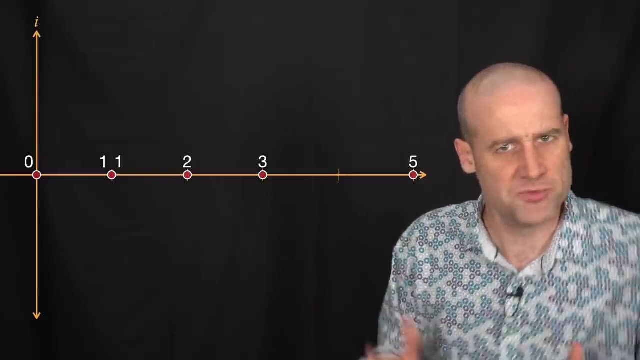 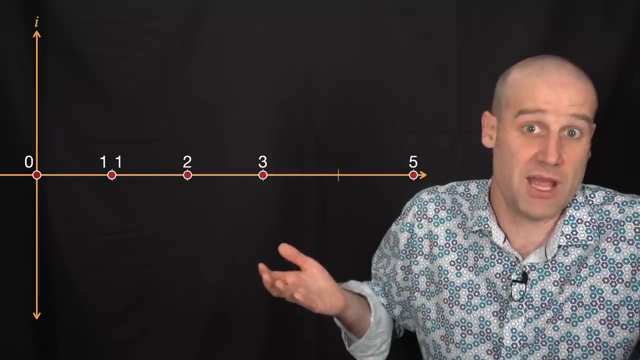 positive real values of n. and so here on the number line I've marked the whole number Fibonacci values. we already know those and somehow we're gonna have to go from zero. we're gonna have to hit one twice and then hit all the other ones going up. okay, we'll see what happens. so I coded up the binay formula in: 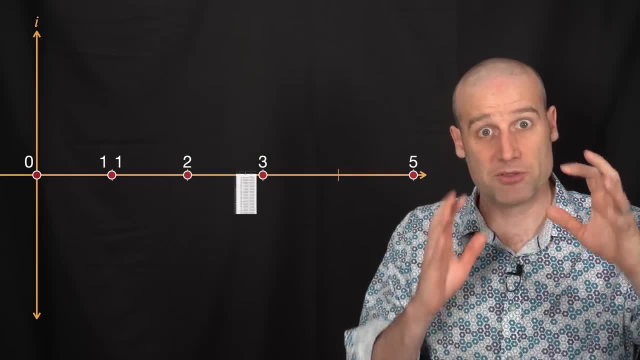 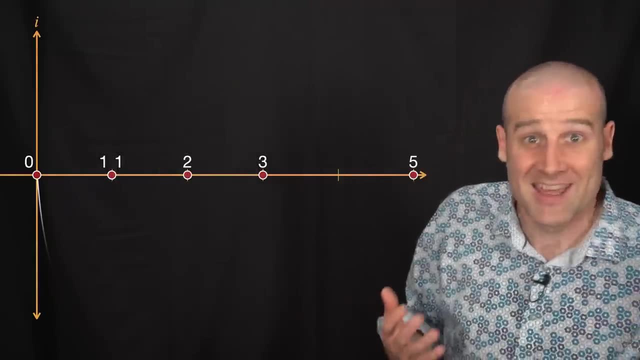 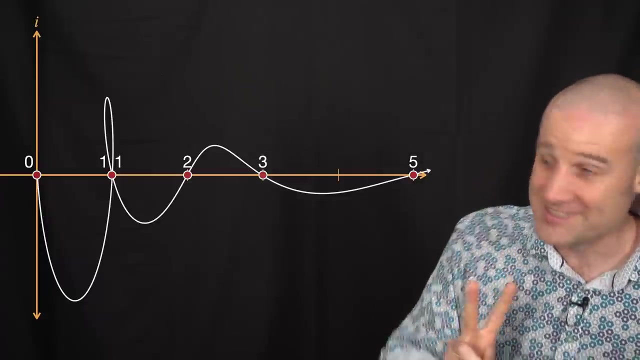 python, because you can use that to handle complex numbers. I then put the real and complex values out into excel and I used it to plot the function and this is what I got. look at that. it does a loop to loop, so it goes through one twice. it gives this: 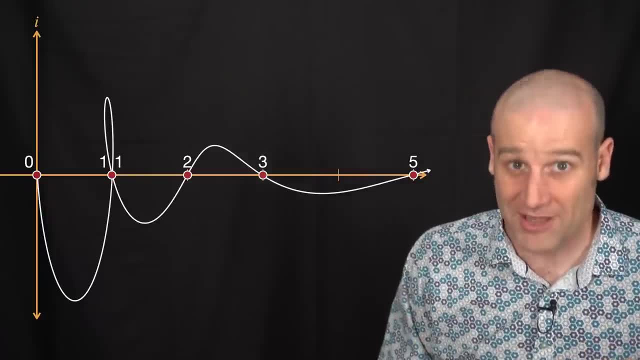 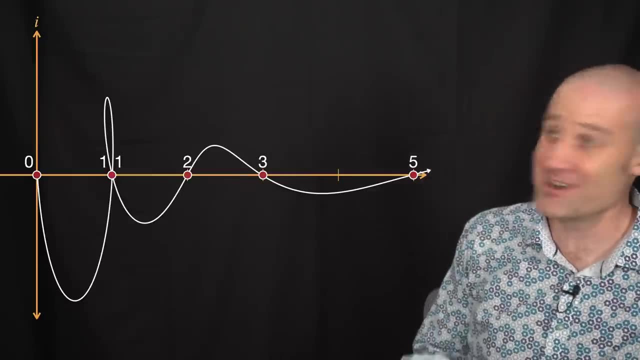 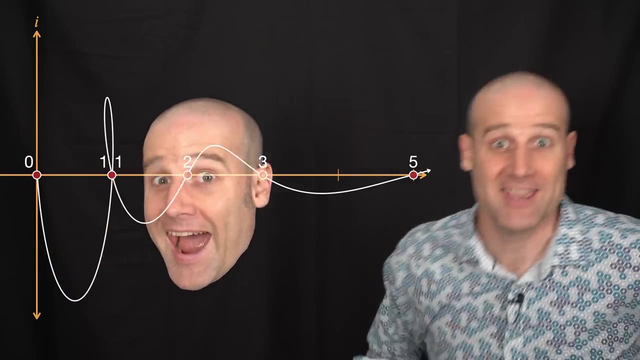 fantastic line. these are complex values and whenever they cross the real line you get a whole number Fibonacci. when I first saw that, I just tell you what I very quickly had to find: my amazed face and oh, oh, okay, here it comes ready. this is what I look like. 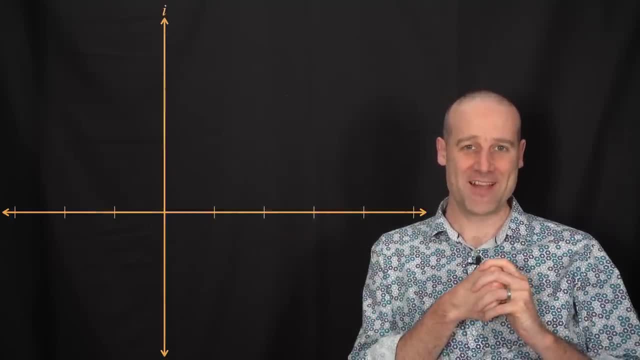 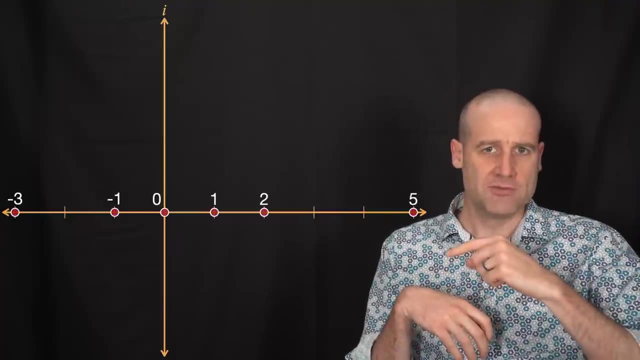 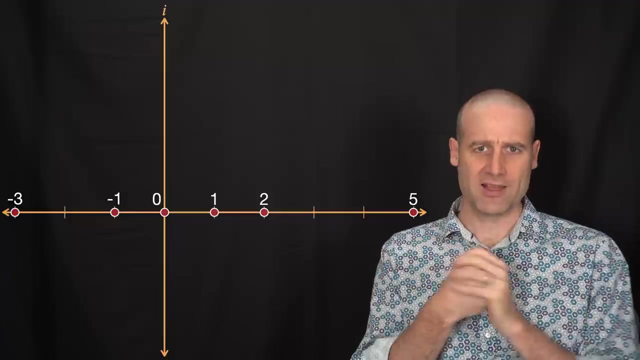 amazing. and of course we can do the negative values of n. interestingly, this is going to have to skip backwards and forwards between positive and negative whole real values. so sure enough, you start putting in the negative values of n into the binay formula and you get a spiral. that's how. 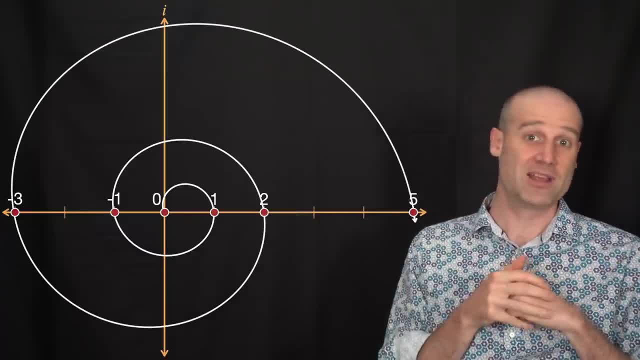 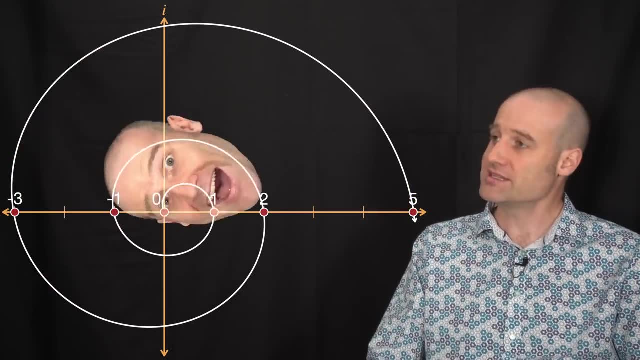 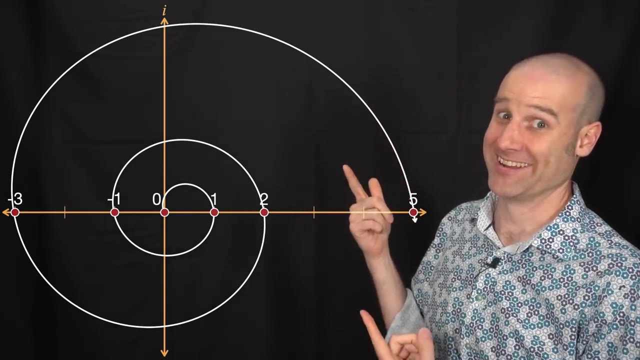 it skips backwards and forwards, and every single time it hits the real axis it always crosses it at a whole number. it's: oh, oh, I guess we're we're doing the amazed face thing again, though that's fine. it is pretty amazing, so ready, amazing. for the record, these are not the same scale on the vertical axis. these are my actual. 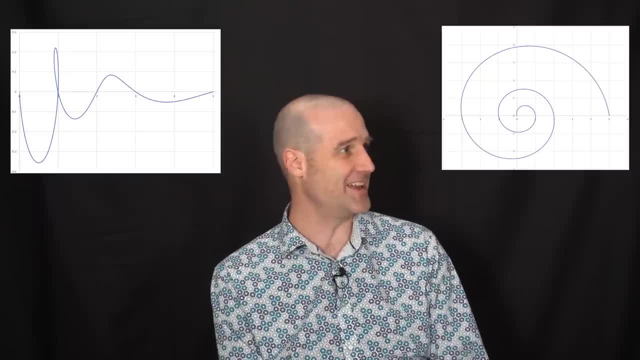 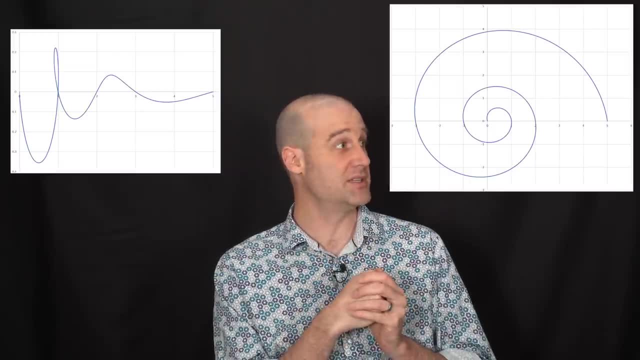 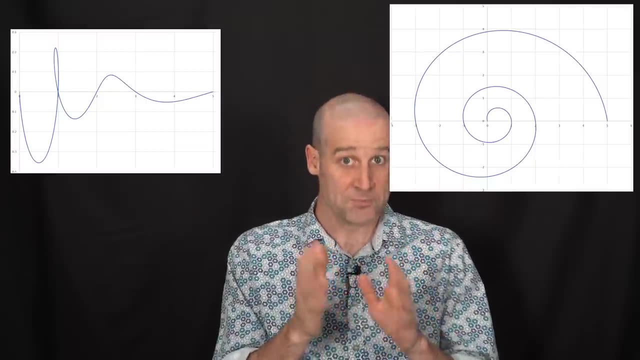 original excel plots, not made to look fancy or anything. and for the negative value of n one it is the same scale in both directions, both for the real and imaginary numbers. this is while plotting the real axis, and at the peak there the imaginary component gets almost up to four, whereas for 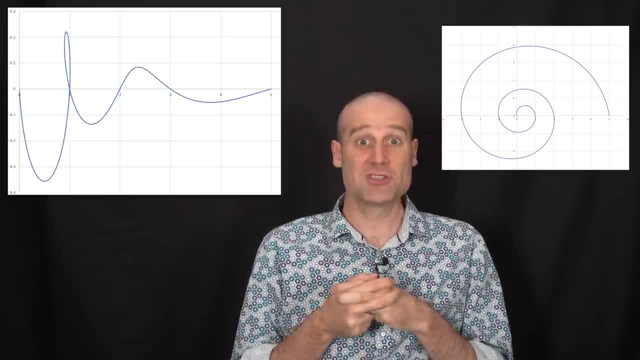 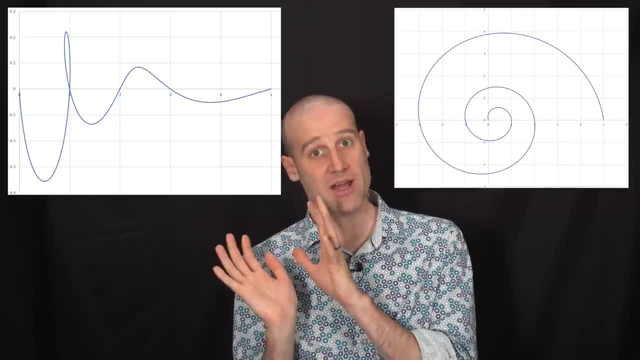 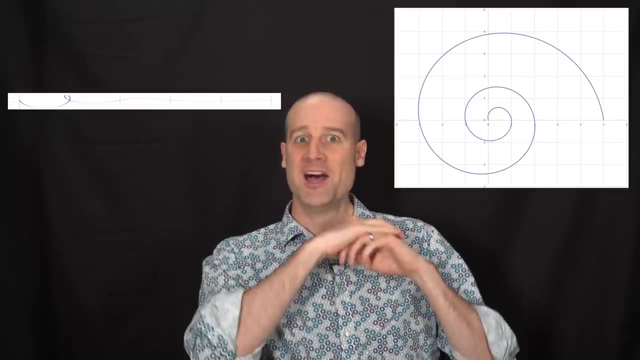 positive values of n, that vertical axis only goes up to just over 0.2. so if you were to plot both of them at the same time, all the details from the positive one are totally lost, right? it's barely going above and beyond the real axis, whereas the nature of the spiral literally spirals out of. 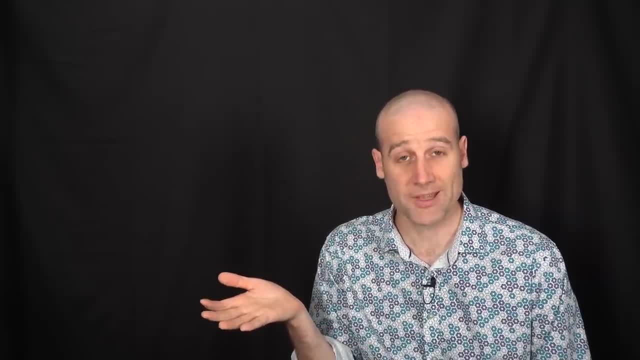 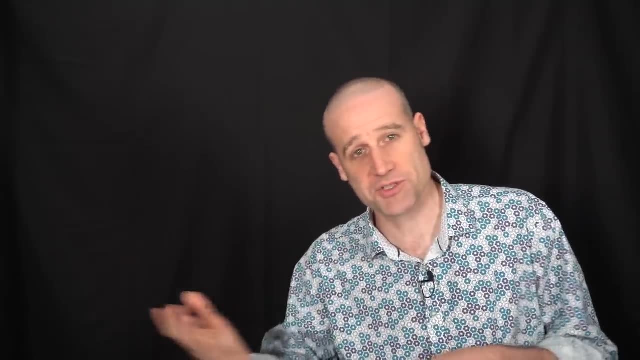 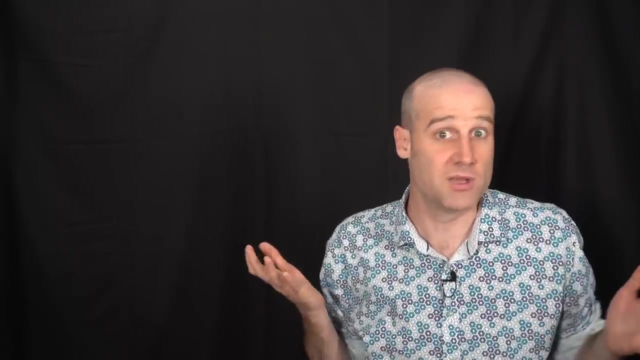 control. fine, we'll do it into a very simple formula if you're putting in a complex value of n, because if we can put in real values of n and get out complex results, what's to stop us putting in complex values of n and nothing mathematical? to be honest, the binet formula works great if you put in complex values of n and look. 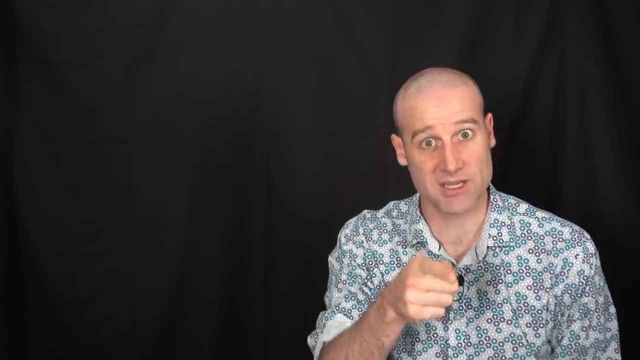 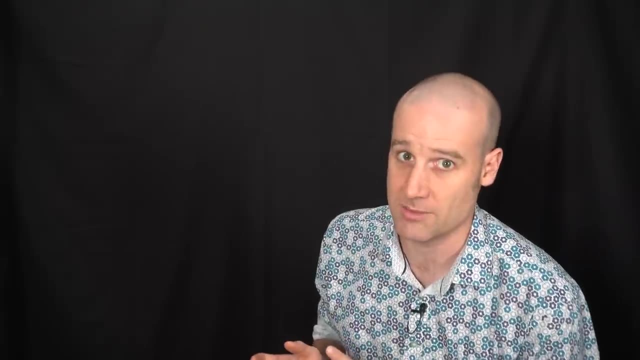 at the complex results you get out. the issue is our brains, because a complex number is effectively a two-dimensional number and if you're putting in a whole range of 2d numbers and getting a different 2d numbers out, that's a four-dimensional plot. to be able to look at all of it at once and as 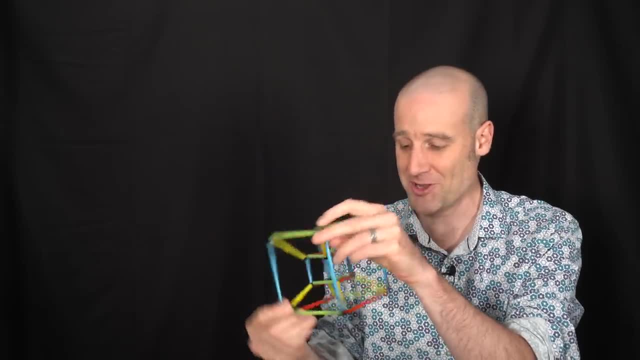 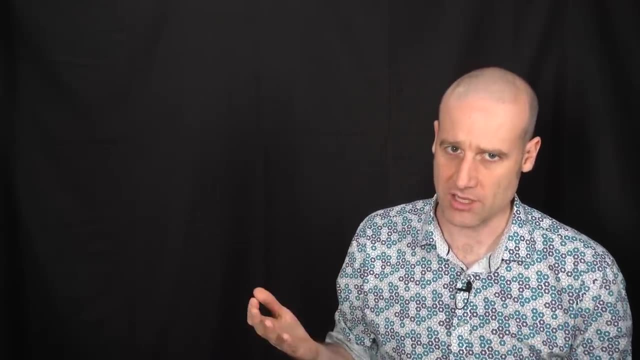 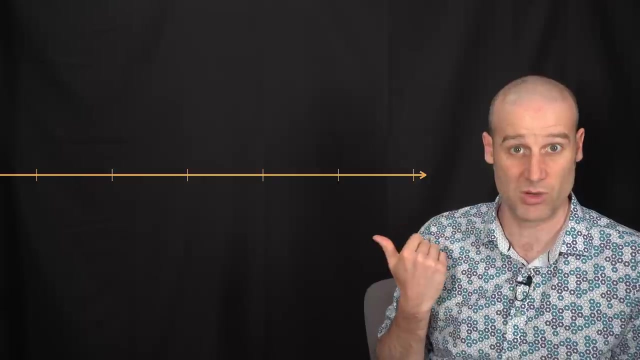 previously discussed. i am a huge fan of four-dimensional objects, but our brains don't play nicely with such things, so there's no easy way to visualize it. we were kind of cheating before by taking a 1d input, which is just the real number line, and then plotting the 2d. 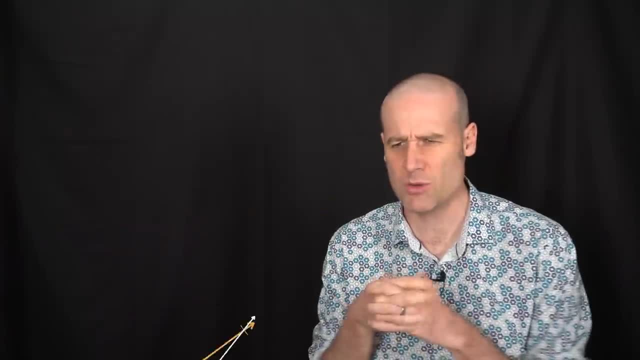 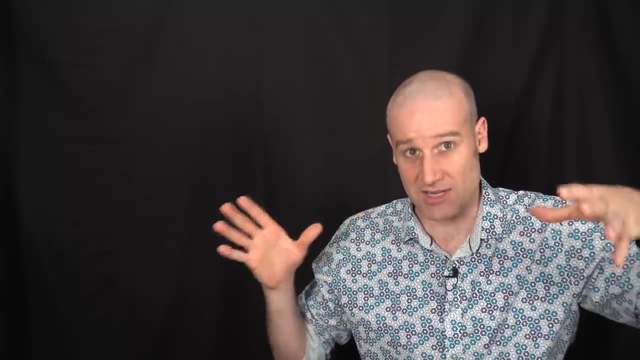 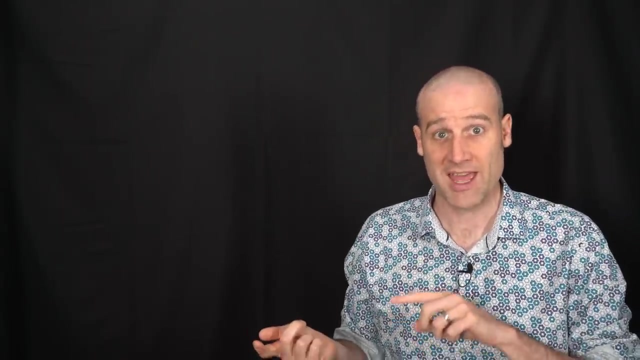 result around it and i started thinking how on earth am i going to visualize this? and what i decided to do was to show all the values of n going in as a two-dimensional surface, the complex plane, and then just look at one component at a time, and initially i thought you know i tried. 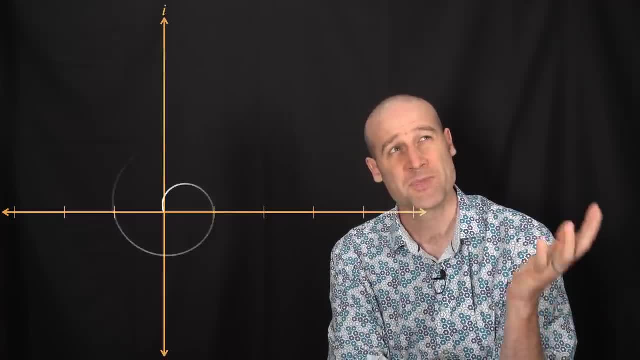 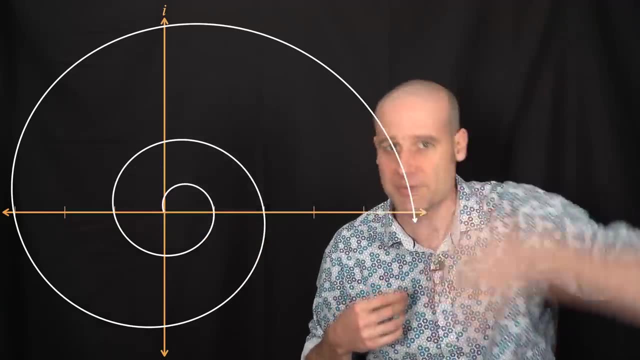 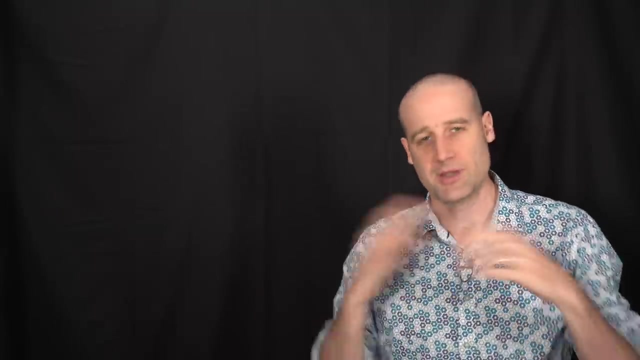 to picture what that's going to look like if you get a spiral. a spiral coming out is both of them oscillating up and down, because the real values going up and down, the imaginary numbers going up and down. so i knew i should kind of see waves in the result. so once again i fired up python, i put the numbers into excel, i tried to. 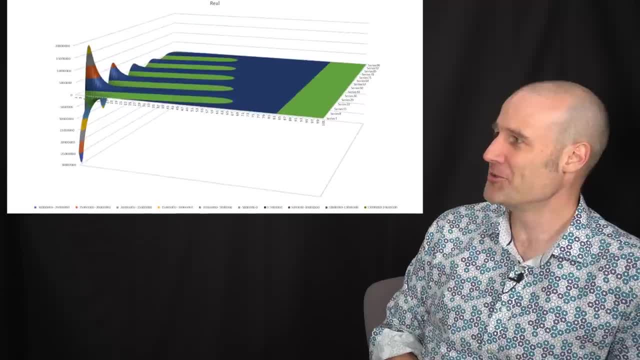 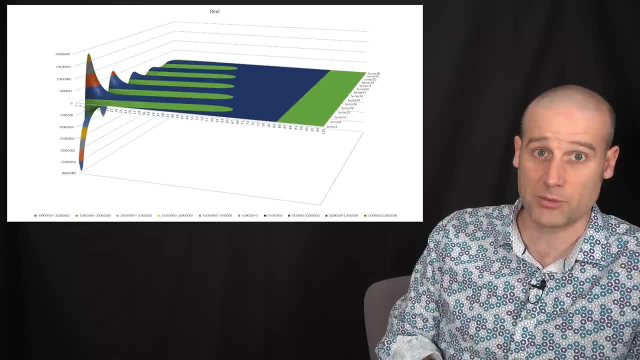 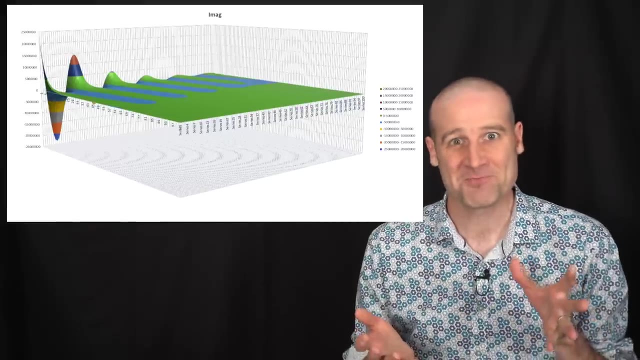 plot them using the built-in excel 3d plots. there you are. that's the real component of all the values that come out of the bernay formula. if you put in complex values of n and here's all the imaginary components, so yeah, you can kind of see that wavy effect. 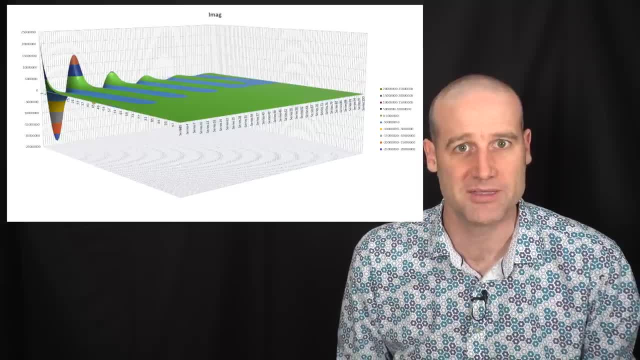 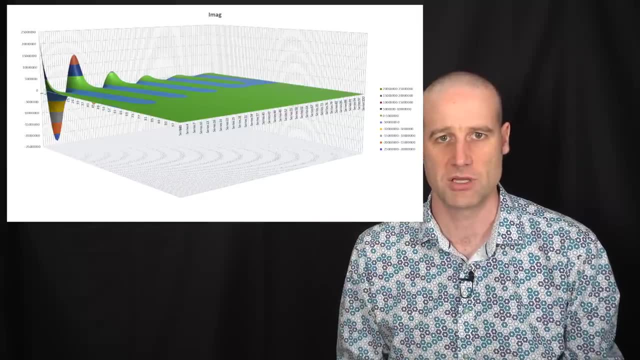 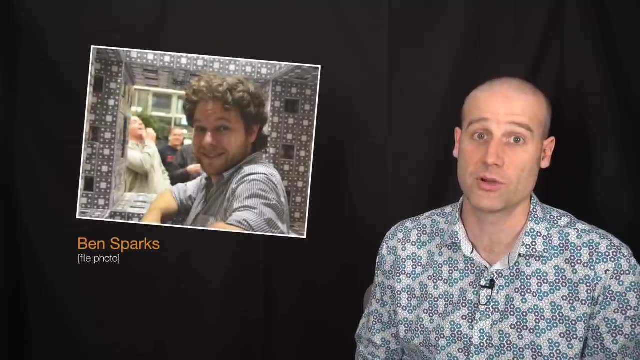 but it's not very easy to explore. at this point i realized i'd reached the limit of me trying to cobble together bad python code with the bad built-in visualizations in excel, so i got rid of all of that. i contacted my friend ben sparks, who you may know from various number file videos. 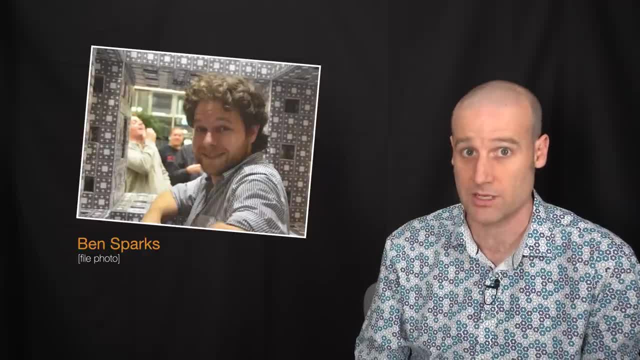 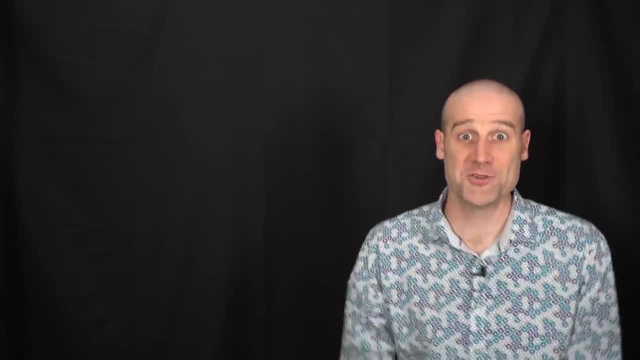 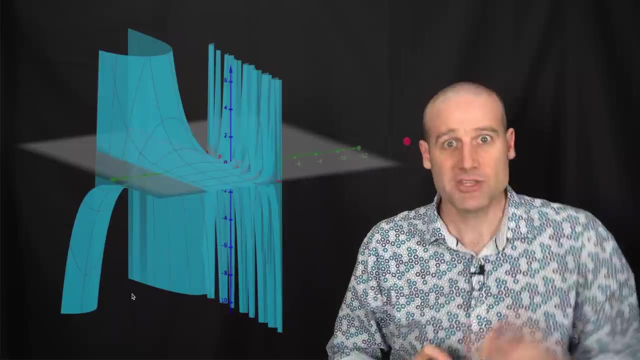 and other fantastic things that ben does. i work with ben a lot doing mass communication work and ben is an absolute ninja when it comes to using geogebra. of course ben could do it, but i couldn't and geogebra he made this right. so this is just the imaginary component and again, 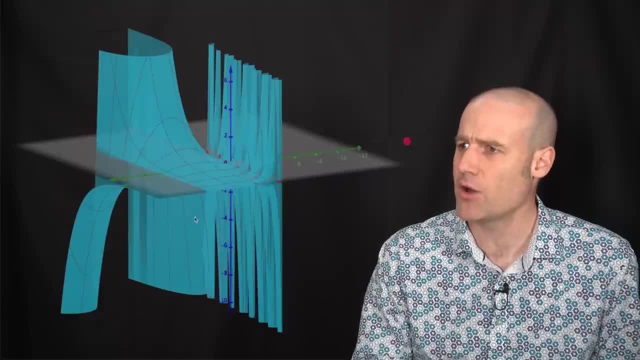 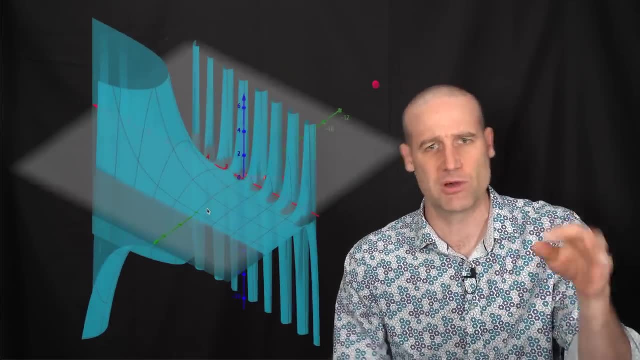 you've got the complex plane for all values of n going in, but now i can grab it and i can move it around. ah, and because we haven't got the issues i was having before in excel, where it was cutting off at weird values. georgia was far better at doing this because it was designed to do it. you. 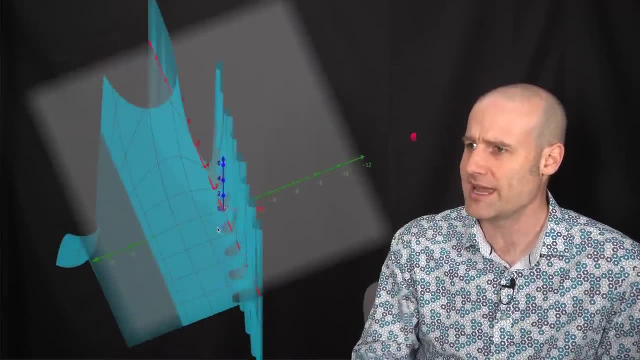 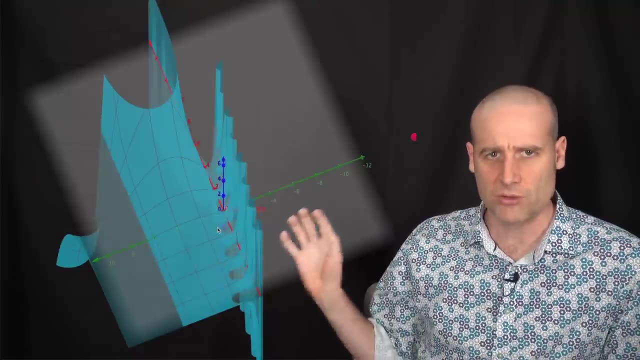 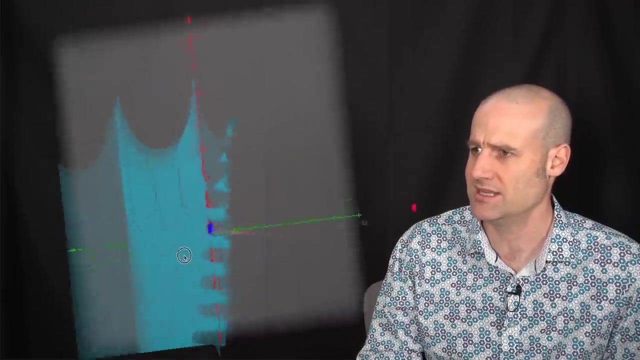 can now move it around, you can see. so there's that red line down the center there, the one that goes here and then kind of goes all the way back up over there, that one there. that is the real number line. so originally that's the only bit we were looking at, and as i twisted around, you can see. 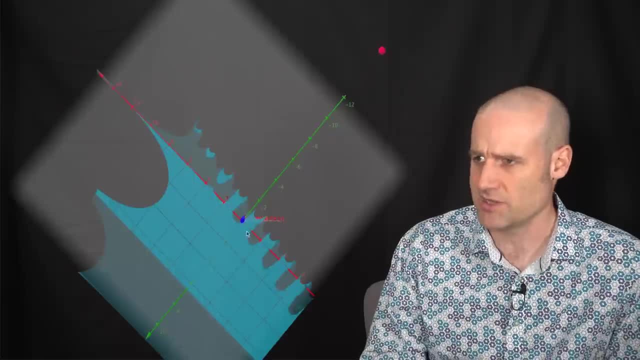 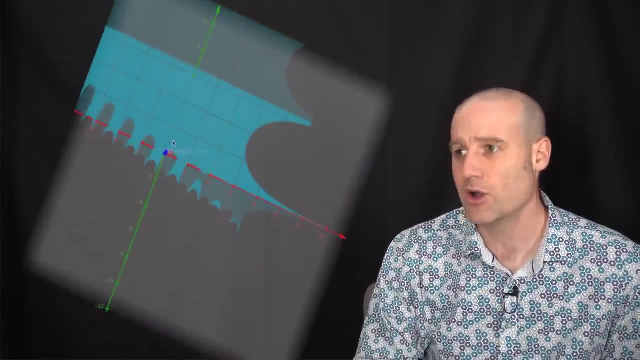 there there's the kind of: this is the negative direction over here. so that's where you get the undulating up and down complex value that forms the spiral, and then in this direction over here, that- oh, this is kind of cool, you can see these- um, the undulation goes off and so by the time you're 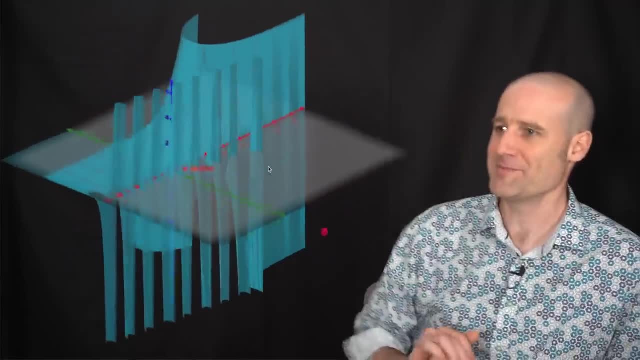 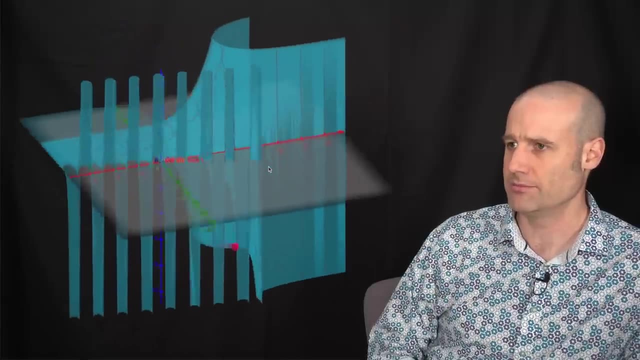 over here at the positive values, you're: um, oh, look at that, i made it spin. look at that. then you get the bits where you get, like that, loop to loop, but then it carries on for ages just ducking above and below, um, the real line, and you 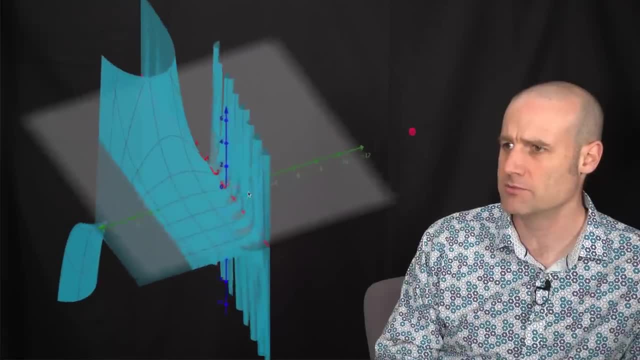 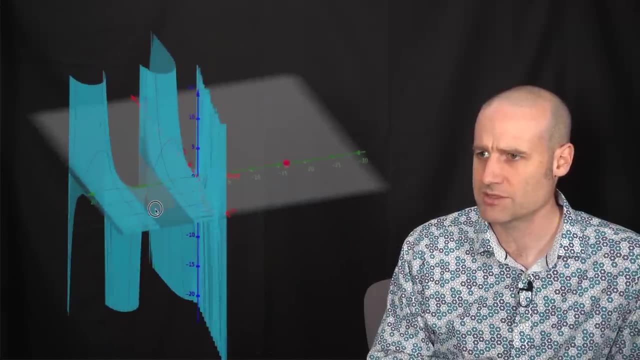 don't have to stop here if i stop that from spinning. we should be able to zoom out so we can see more of it at once. so wrong way, here we go, out, out, out. so look at these. you start to get these things like: what's going on? there's another one of these, where'd that come from? so if we zoom back, 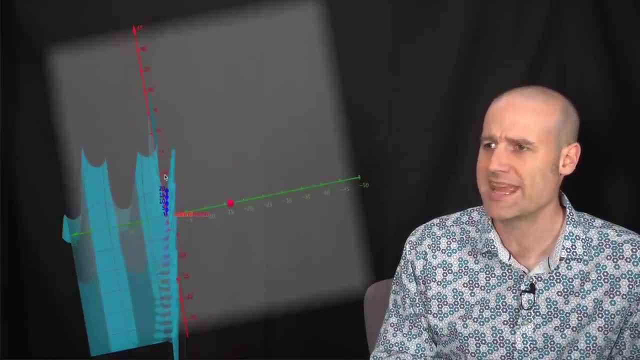 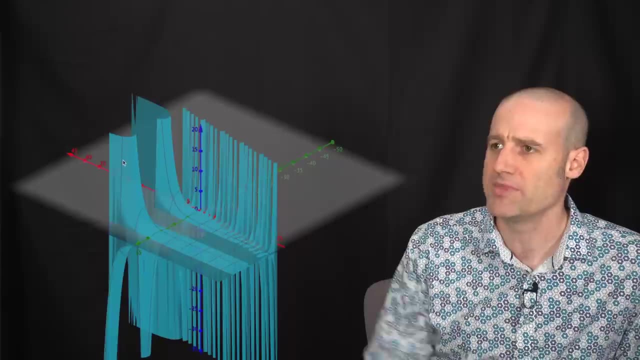 in fact there are more of them and you can see they line up. that's um. if you can see that's 10, uh, positive 10 on the real number line up there. you get these ones where they get these huge spikes and they don't stop at the top there. 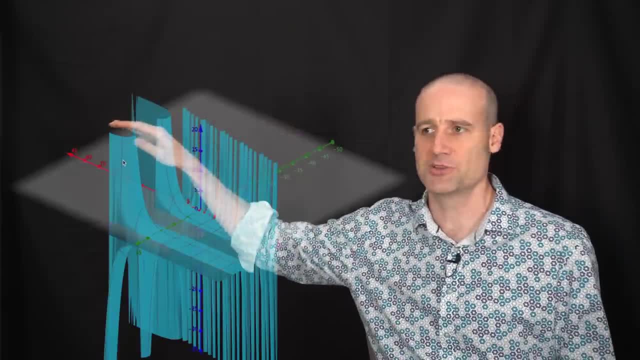 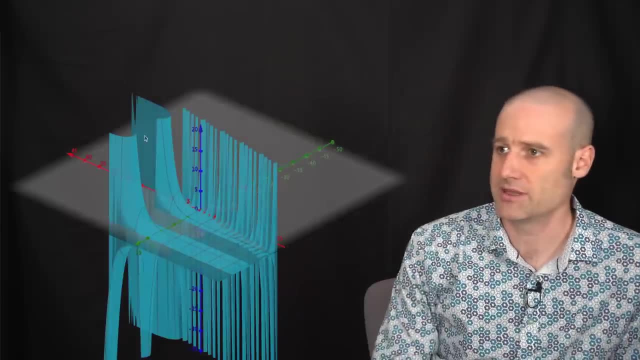 by the way, so that, um, that you can see, the top here looks like they kind of cap out. they've not capped out. that's just where georgia was limiting how far it was drawing, so it's not drawing everything above that. uh, you can see they go. oh, they go off in the? um other direction underneath. 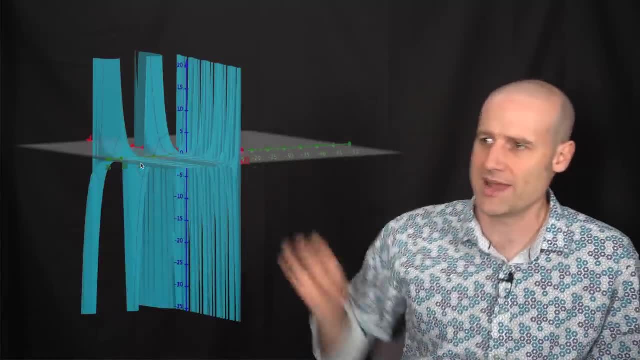 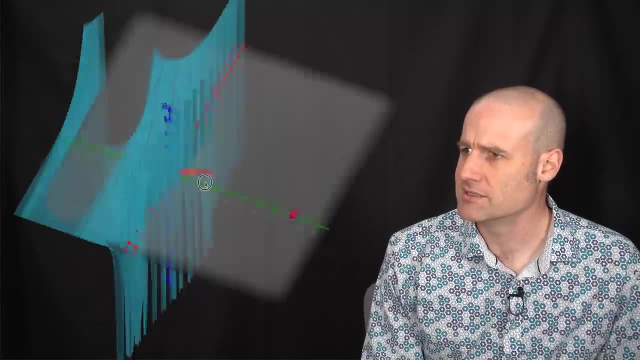 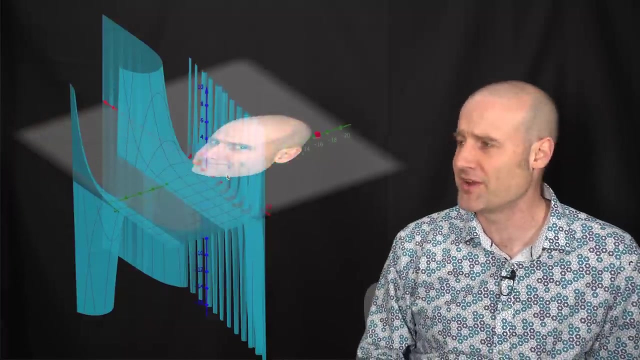 you can see here they start really low and they come racing up and then they curl around out onto the ah, so cool, and so i don't know what's going on over there. that's kind of fun. i'm going to zoom again so you can see us. let me just: ah, i was very impressed and oh, look, it's my very impressed face. 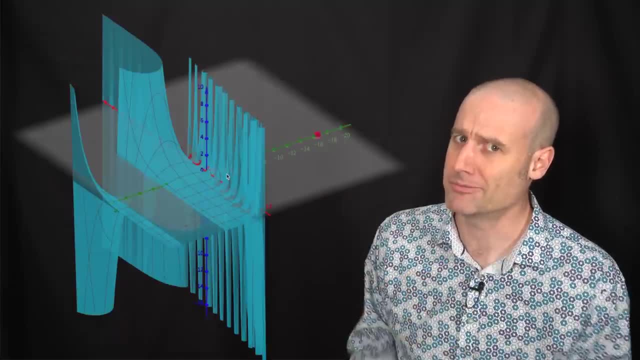 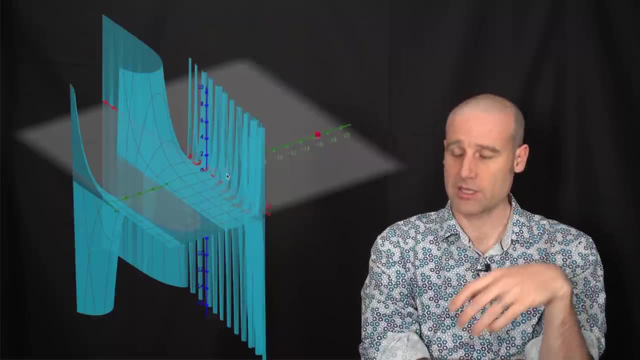 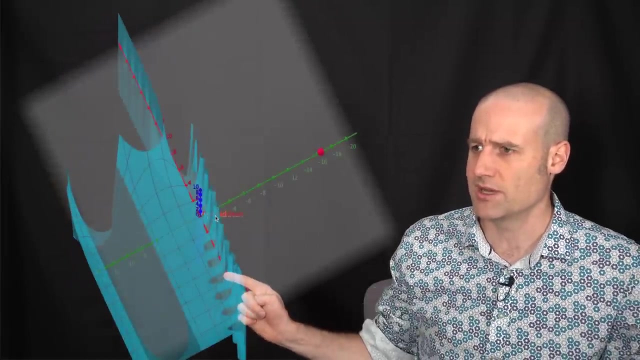 ready, very impressed. this does open up yet another way of exploring this four-dimensional plot that we unfortunately cannot visualize. and, like i said so, we were looking before at the slice down that real number line, so the red line that goes all the way back along. there we were just 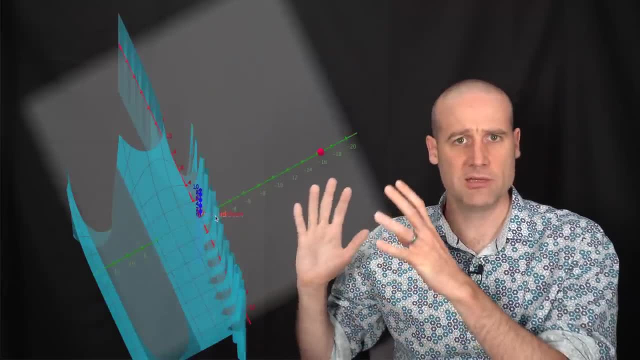 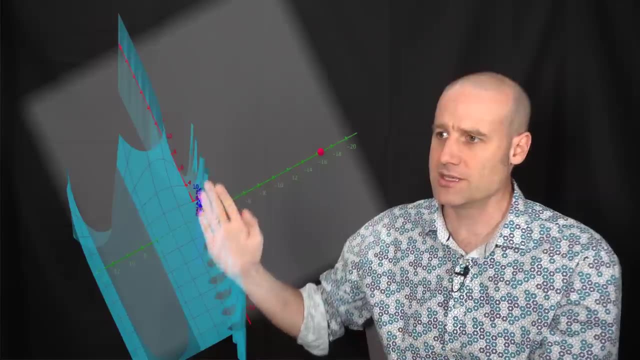 taking that as the input and then looking at the 2d complex plot that comes out of it. but why don't we pick a different line? in fact, we could choose. we could, instead of choosing that, we could increase the imaginary value. right. and what if we picked a line like uh, one that goes across the complex? 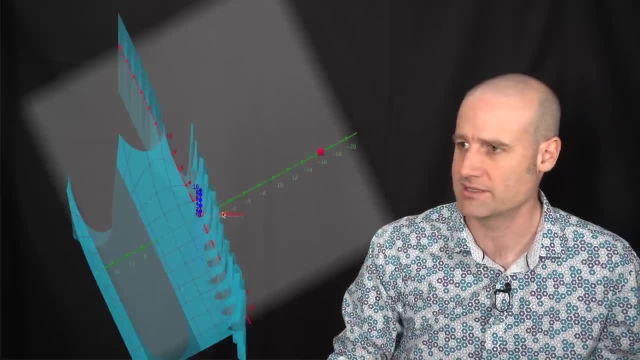 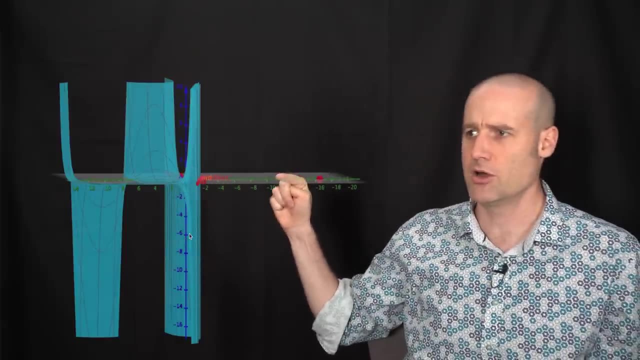 plane over here somewhere, like i don't know. i'm pointing the totally the wrong way. compared to that, you get the idea right. so instead of let me do an end on right, so instead of going along here, why don't we go like along over here somewhere, or along over there somewhere? 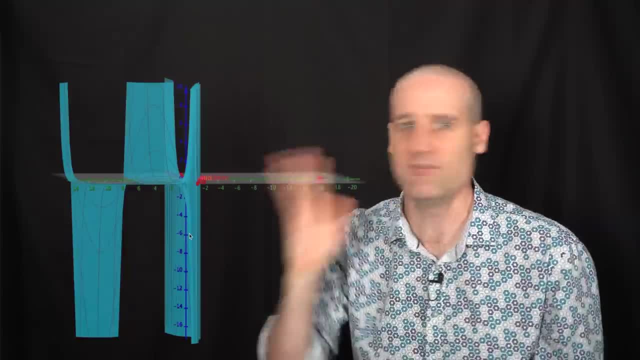 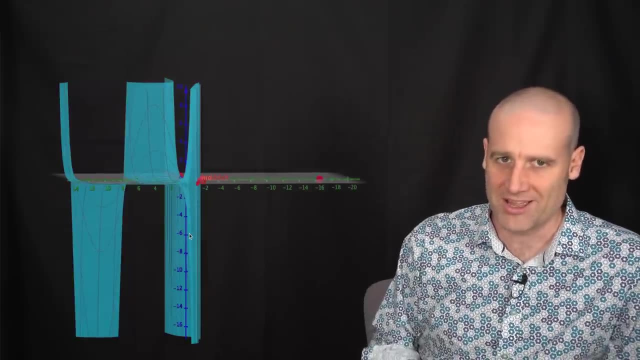 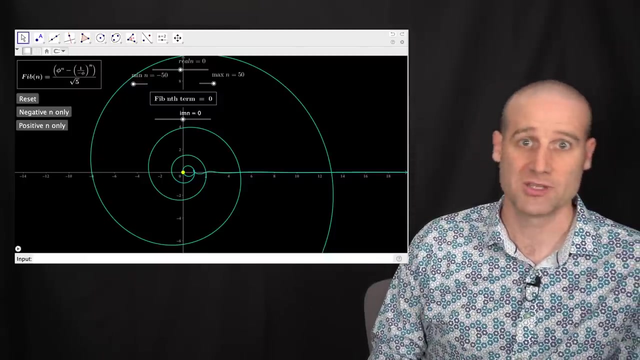 i think this is probably willing to work at at least a bit of a different way. we've already looked at the figs which are on thewan Cosine scrooge poi from another book. but the until i get this, it's going to do it right here and it's easier. I have jpeg on here. 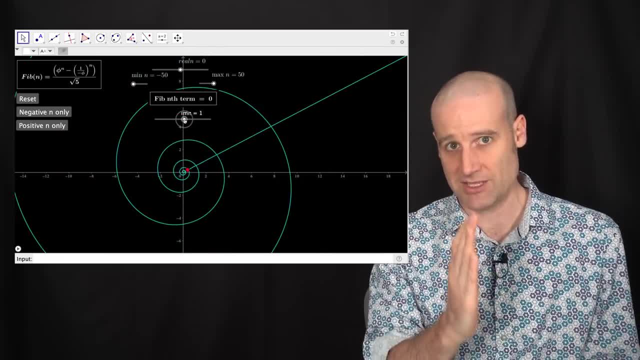 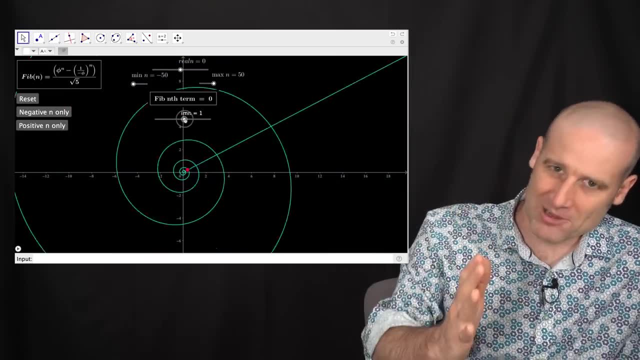 in terms of complexity. amount. jpeg that I used last time. i was also using the qolsq as a argument and what that means is that when you overwrite, you can change type. when you overwrite complex plane staying parallel to the real number line, you can see that the 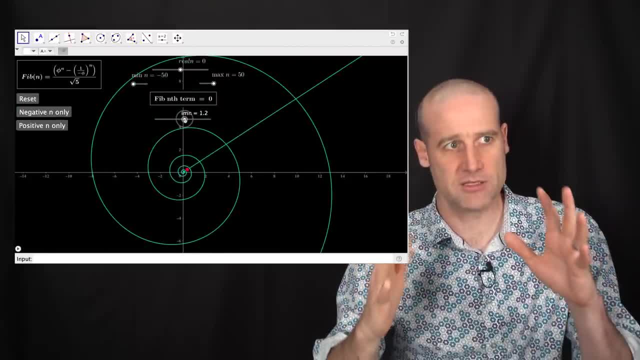 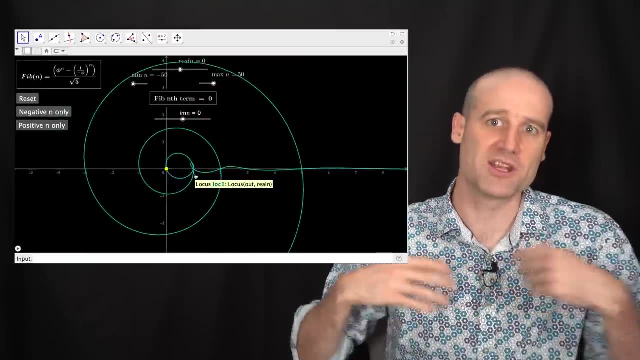 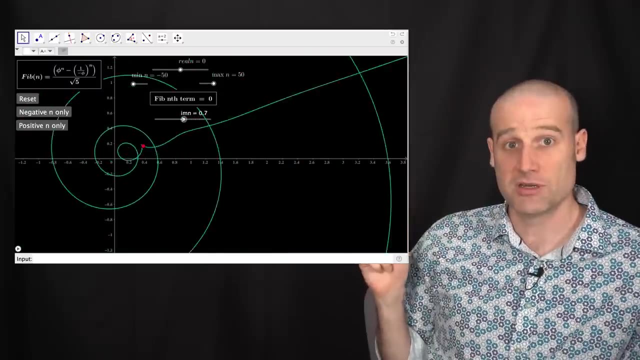 plot changes and so this is a different way of exploring it. we're kind of moving through different 2d cross sections of the plot and you could have more exotic lines which aren't parallel to the real number line. but you can work that out yourself. Ben has made this version available for free. I'll put a link in. 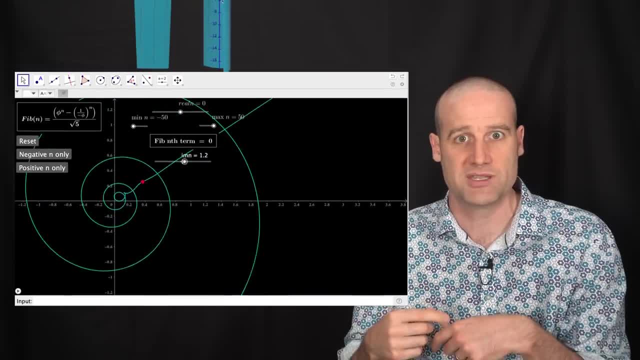 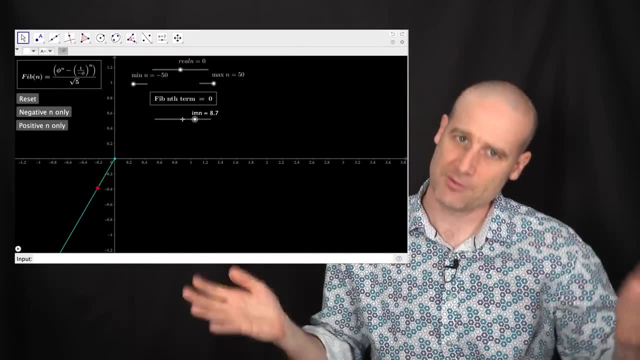 the description, you can get, you get it. and the other plot I was playing with a second ago, yep, that one there and you can, to your heart's content, have a go, and if it looks like things disappear as it before, that's not an actual nature of. 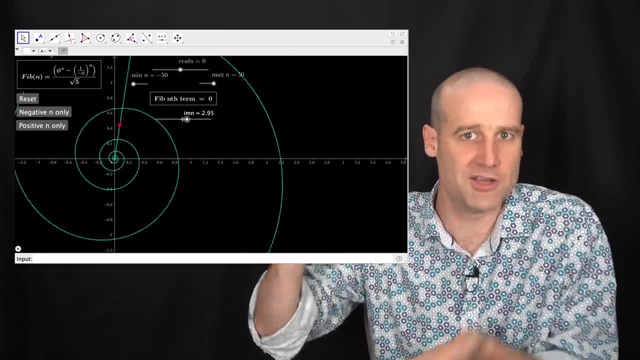 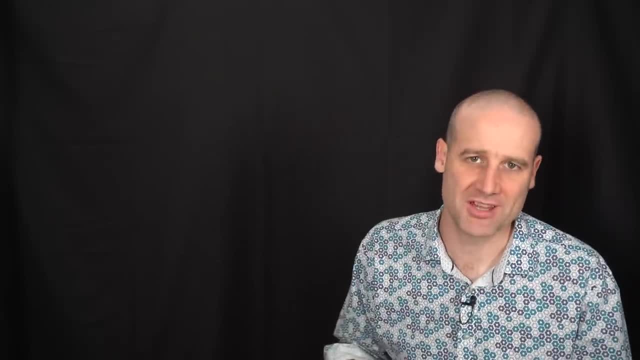 the plot often that's just it's. we had to cap how far Geogebra bothers going, but it's all below download it. have a play quickly. there is another way you can visualize things and that's by just taking the absolute value of the complex number when it comes out, so you can see that the number line is parallel to the real number line. 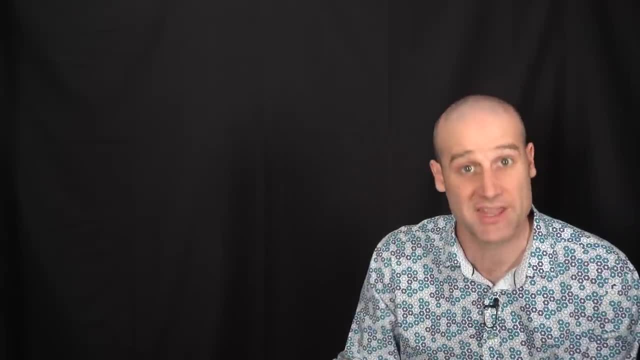 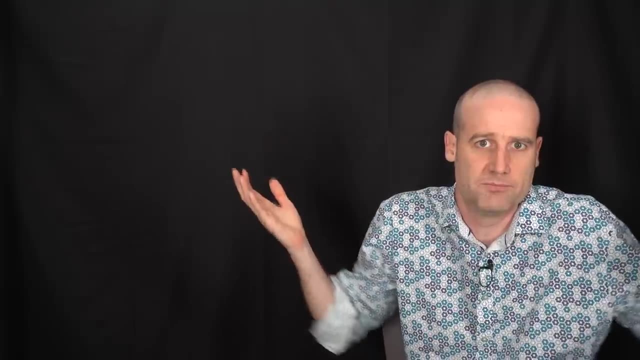 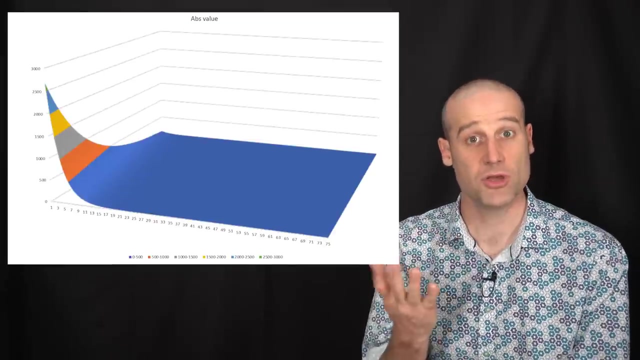 you have the complex plane visualized going in and then just the magnitude of the answer, so you effectively ignore the direction where the complex number is and just as its distance from 0 plus 0i, and I initially tried that in Excel and got a terrible, terrible plot undeterred. I thought I would just filter out and 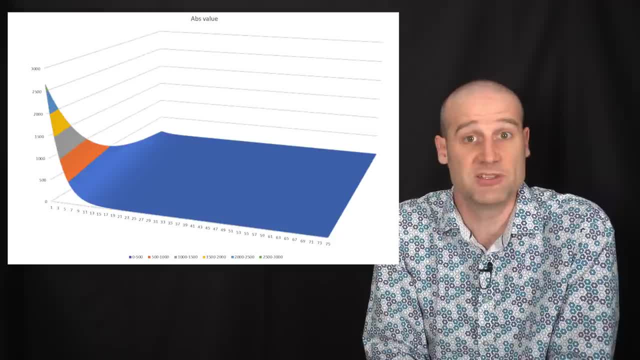 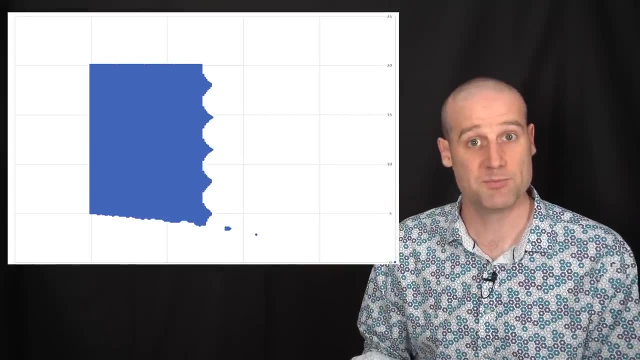 find the interesting bits and for some reason I thought: wouldn't it be fun to look for the zeros? so I did a map of where the lowest values are and I got this. I became a bit obsessed with that little dot by itself and I worked out the exact. 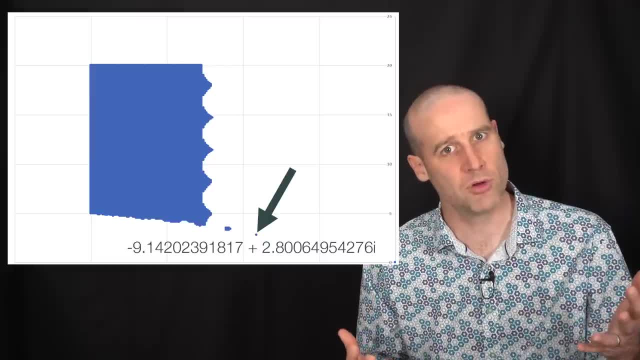 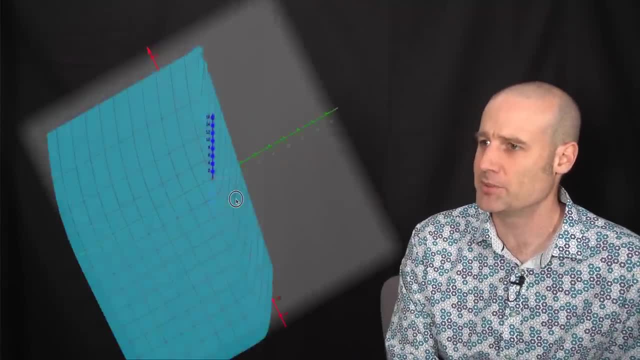 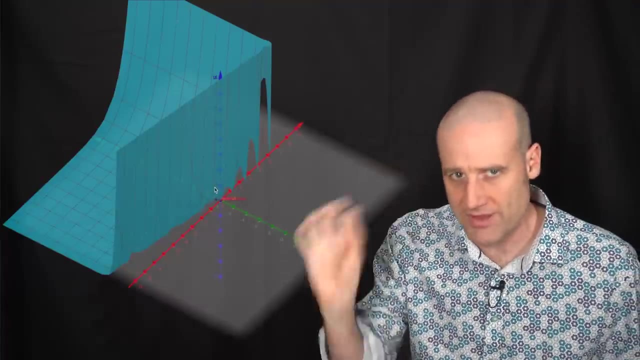 coordinates of where it was, but I thought I wonder if there are more zeros contacted Ben Ben made this for me in Geogebra, so it's another plot. that's the complex plane going in. you still got. the red is the real axis, green is imaginary. this time it's the absolute value of the result that comes out, and what I'm 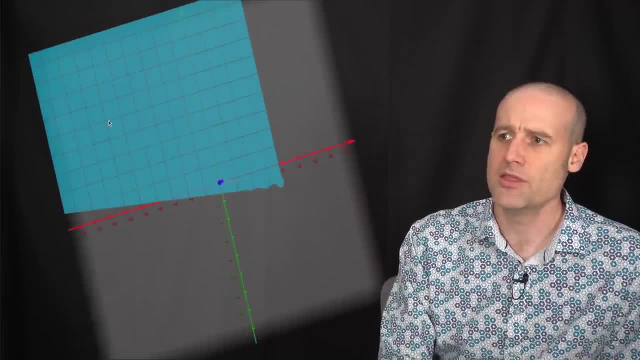 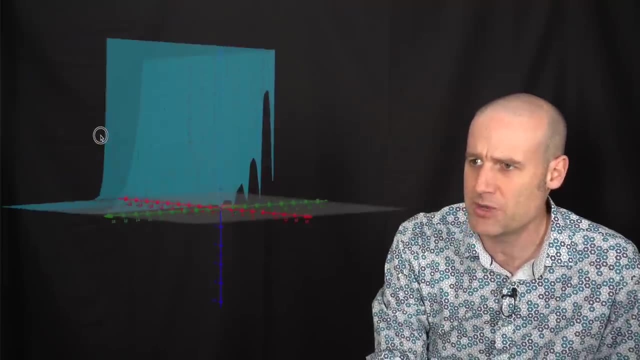 showing you, before you look at it kind of this way, all of this plane, that that whole plane kind of there is super small. so if I angle it down you can see it's. it's pretty much. look at it, it's flat, it's like a sheet. it's just been. 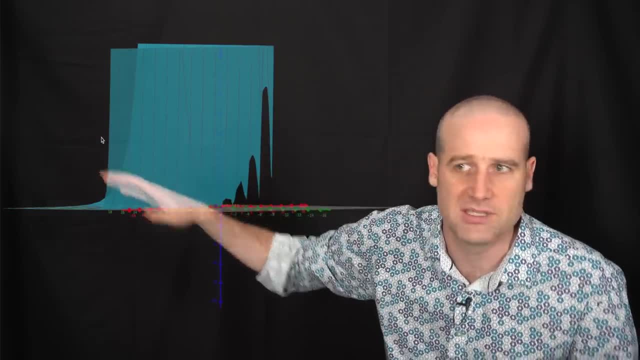 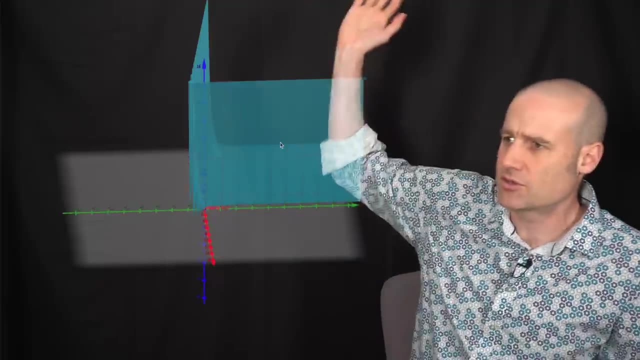 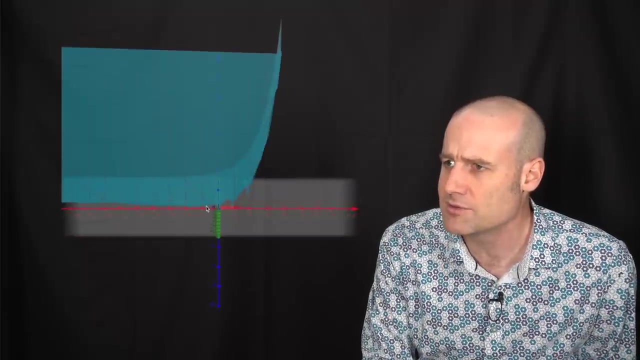 dropped on the complex plane right, so that's like goes off to zero there but then races up massive in both these directions. you get these two kind of aligned, where it just goes straight up, which is phenomenal, and then you've got the zeros. so what I was looking at was all the way in here, if we zoom right in. 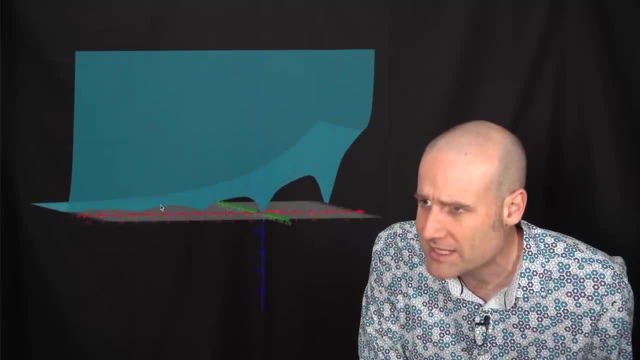 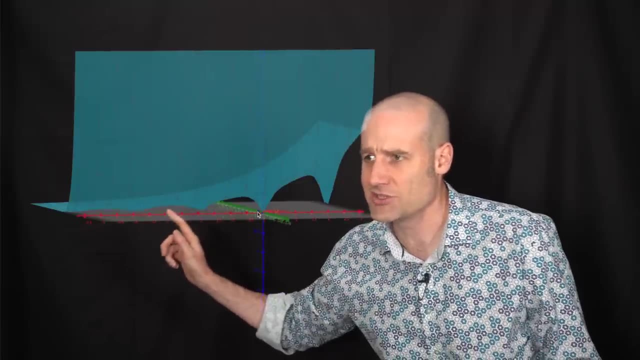 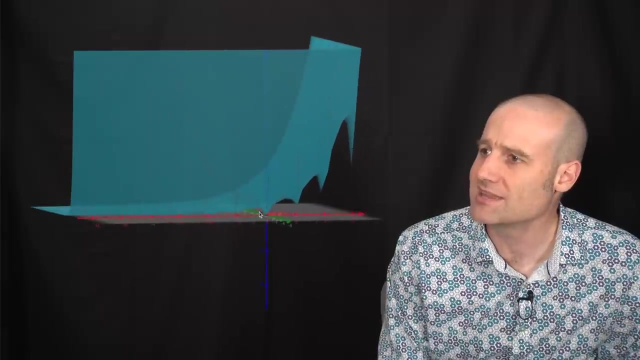 you can just see as it starts to lift up off the plane. it touches and then touches, and then these are. so it touches there and it touches again just about there, and then there, and then there, and as you zoom out it keeps doing that and it looks like these ones that we've just seen, these ones out here. it looks like. 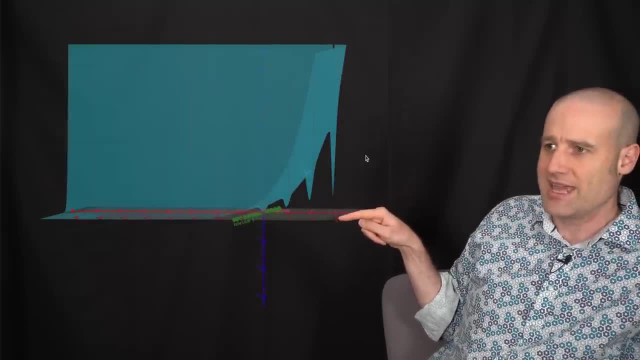 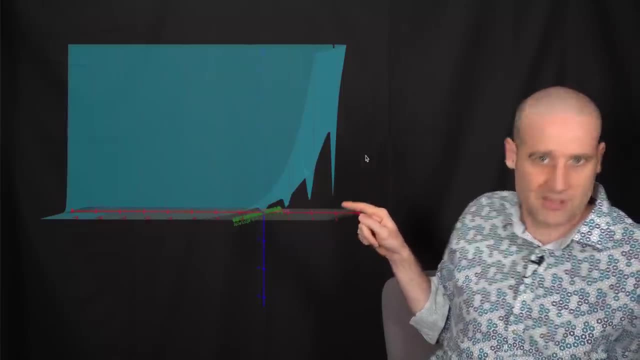 there's a wee gap there where it doesn't quite touch the axis. that's just the resolution. if you zoom right in, or if Geogebra higher resolution processing- because this is just on the fly trying to visualize it- for us that would just continue down. it's too skinny to see and 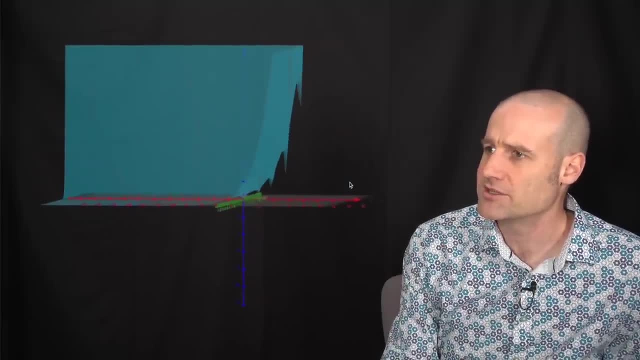 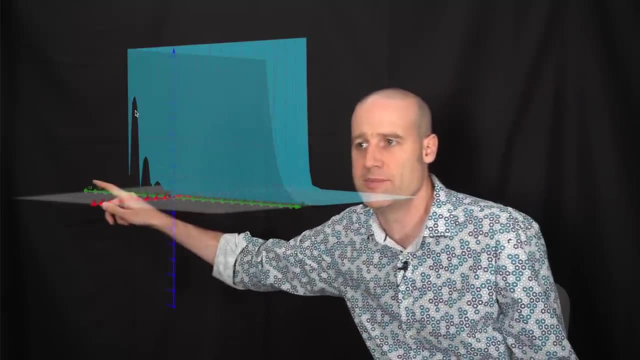 hit the axis and as you zoom, oops, the wrong way, further and further out, all of these, they keep uh, heading down and all of them touch the axis and, and there's like a whole lot of them, no, they're there, they're there, they're there. I. 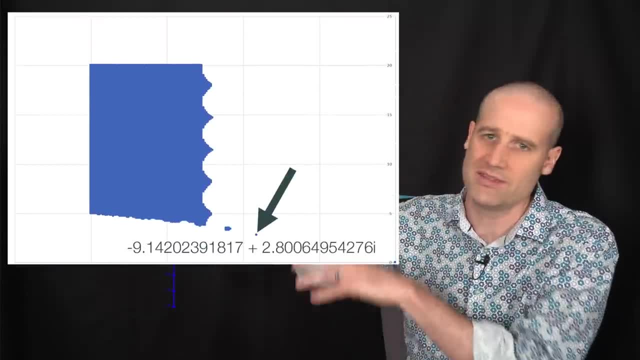 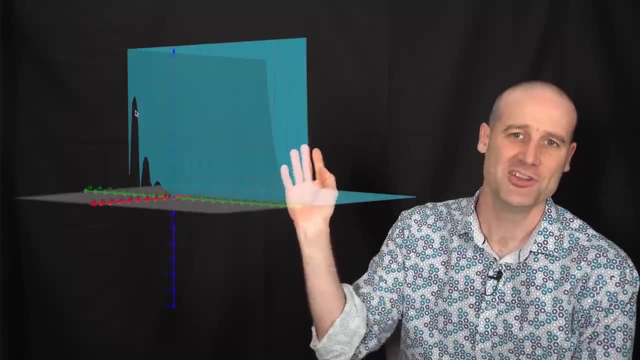 actually then use wolfram Alpha to solve for the zeros, and they're all in a dead straight line there. I think there's definitely many of them. there's a lot of fun with that. so, anyway, this is just to say you can have a lot of fun with mathematics. so I started off by thinking: I wonder what happens if we 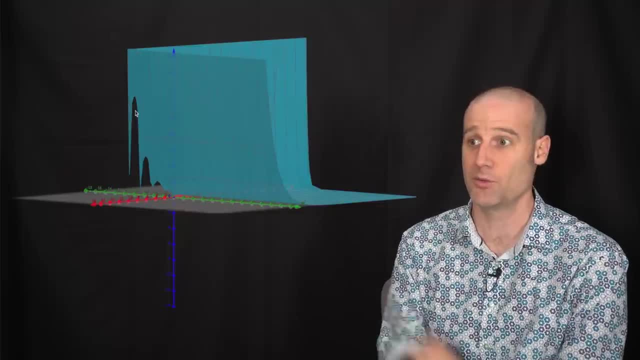 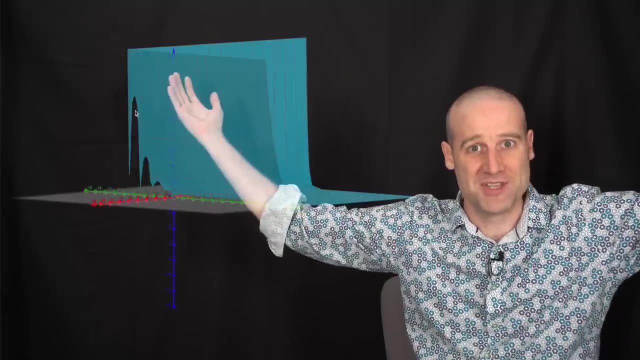 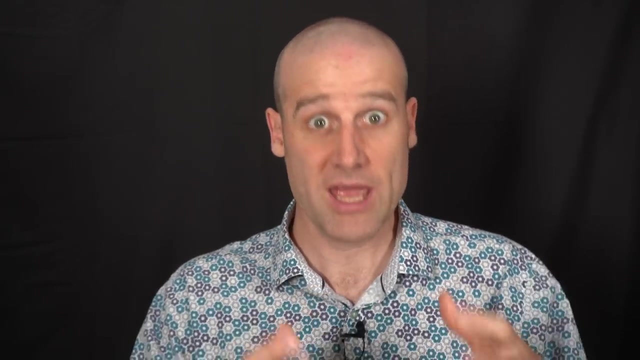 extend the Fibonacci numbers and I ended up exploring where weird zeros are in a four-dimensional plot of the bernay functions. who knows where maths will take you? well, I know a few places. before I say goodbye, I've got two last things to show you that both answer the where can you end up by following mathematics? 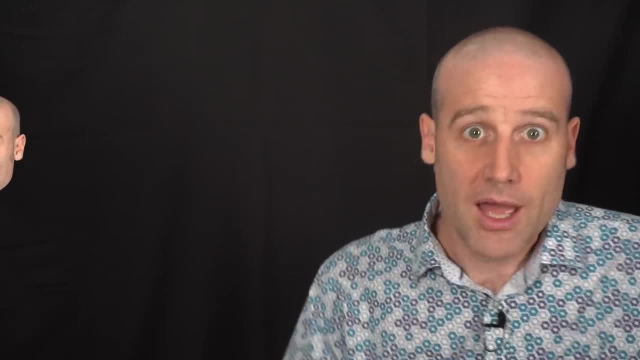 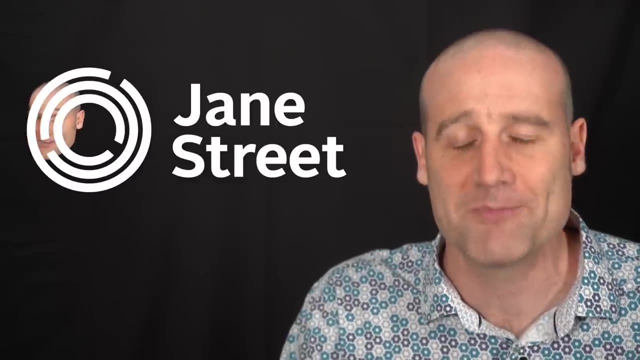 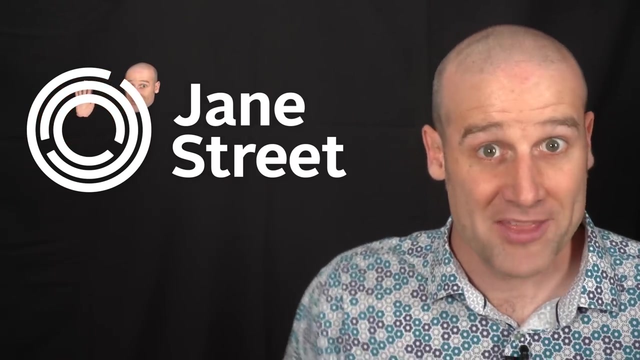 question. and oh actually- and there's my goodbye face- I better hurry up. so, first of all, this video is sponsored by Jane Street. they are, of course, the principal sponsor of my stand-up maths channel and if you enjoy mathematics, you enjoy problem solving and you're looking for a job, then Jane Street might be for you. they. 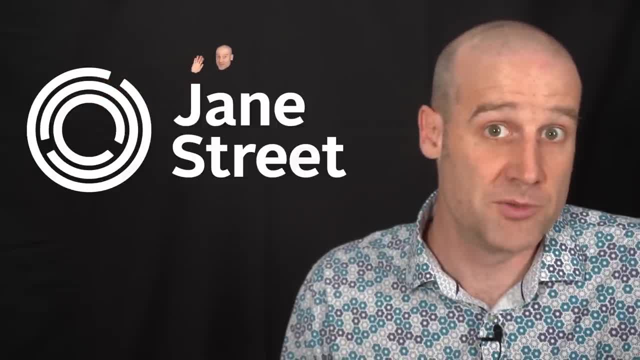 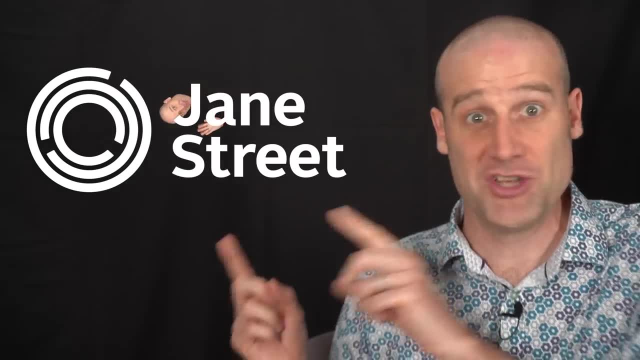 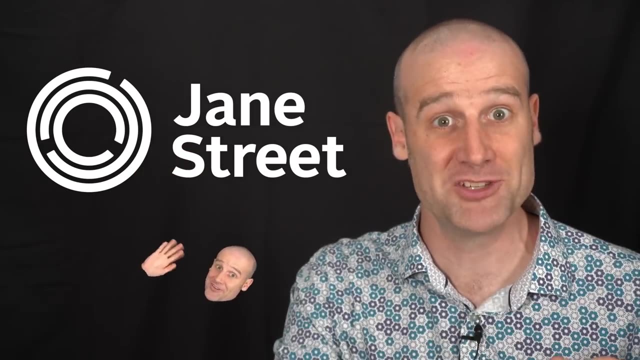 use incredible bits of mathematics to solve complex problems in the financial world. so if this is the kind of stuff you're into and you're looking for gainful employment, then, Jane Street, they support my channel. I think they're great. do check them out for everyone else. just appreciate the fact that they support my